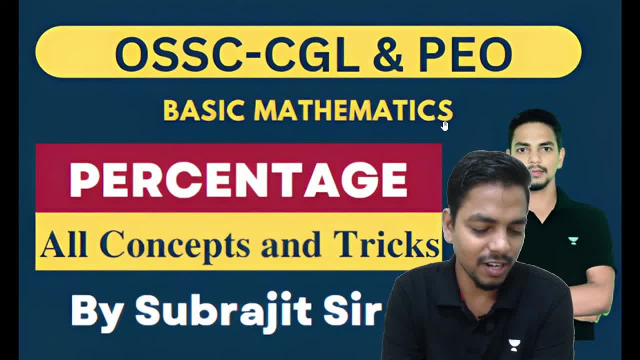 I was thankful that I could leave. So Thank you so much. Naik Nilex Satish, Jyotirmai Subbalakshmi, Deeptimai Smita Sagarika. welcome everyone and welcome to the session. 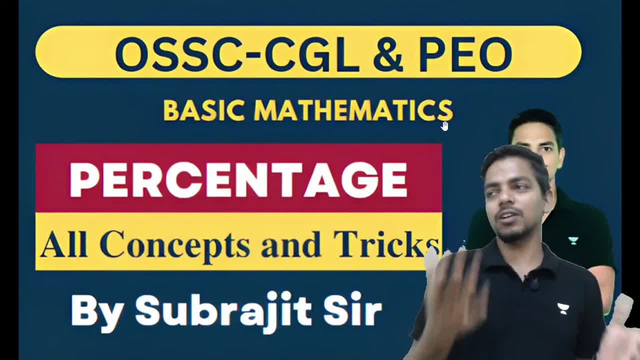 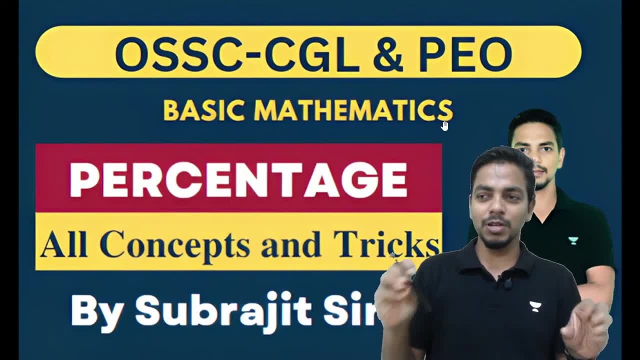 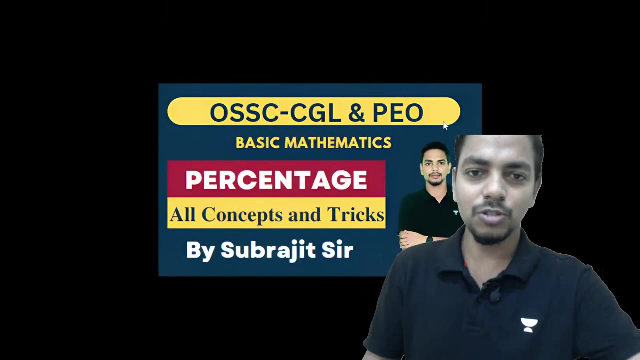 As we all know, if you start with a percentage, you will get a lot of results. You will get a lot of results, But in the current technology world, there are so many applications. If you do this, you will get a lot of results. 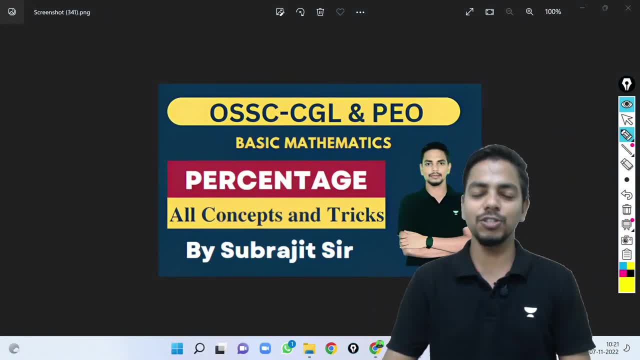 Look at this. So if you think that technology will not be like this, if you write 62% love each other on the top of a technology, it will not be like this. If I give you the number of positive results, it will be 27% love each other. 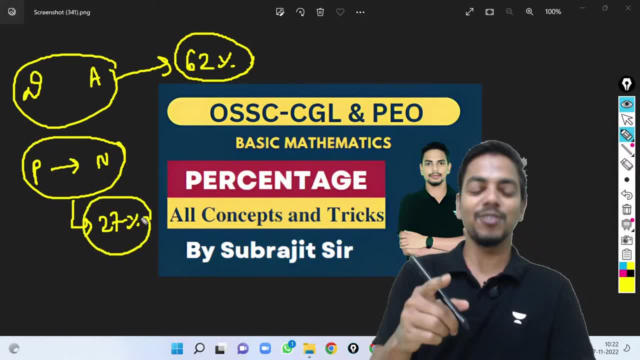 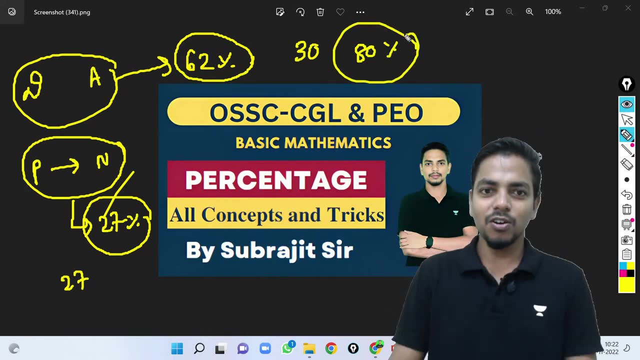 love each other. Love calculator. that's it. that's it. AKM official. this is completely updated. listen to it. If you give it to a friend, then I will give you 27%, 30% or 80%. Who doesn't love each other? 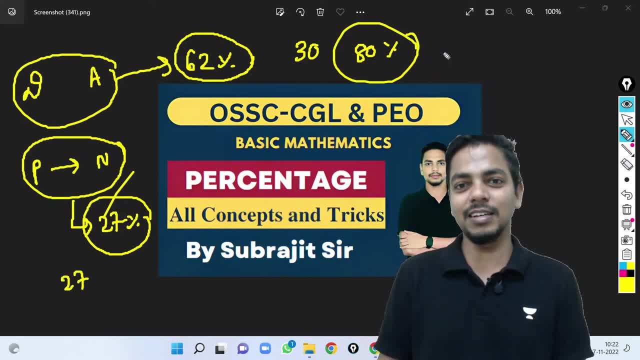 If you look at it, where did it come from? 98%, Tell me. Oh, my father loves me so much, Tell me. and if I give a second time, then the second team gets ten percent. You know it's over over. 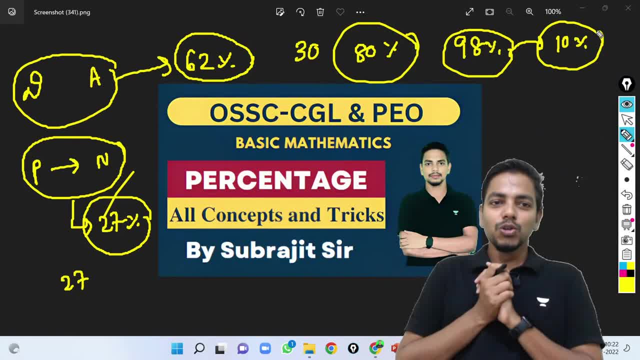 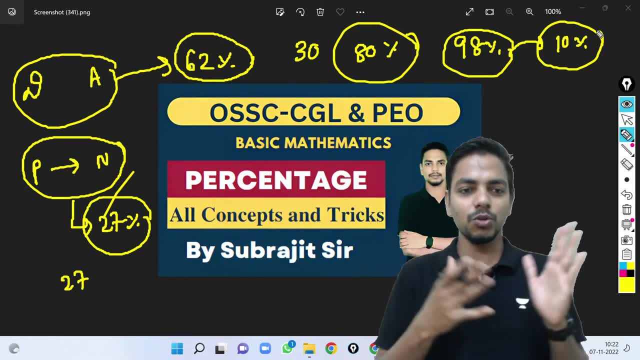 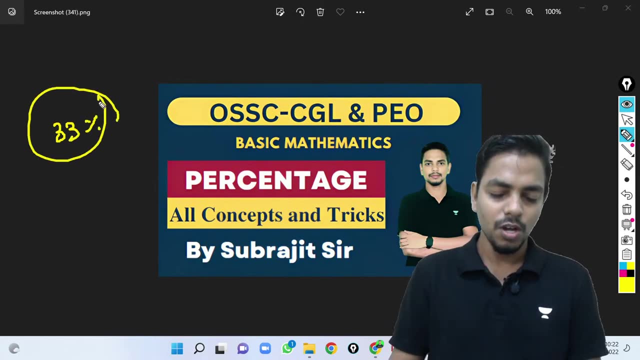 Yes, that's it. So today we will tell you what percentage it is: Ten percent, eighty percent, sixty two percent, twenty seven percent, if you want to give your exam, or to your thirty three percent, you ask for five, I will tell you what percentage it is. 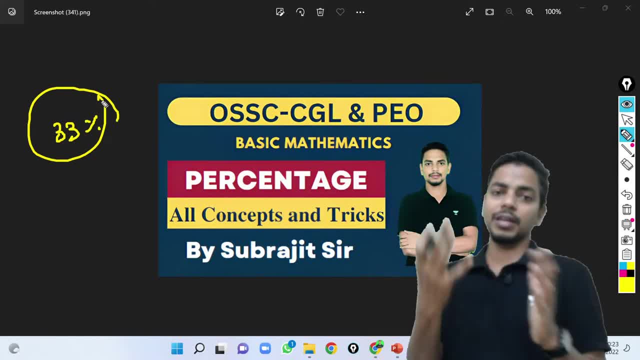 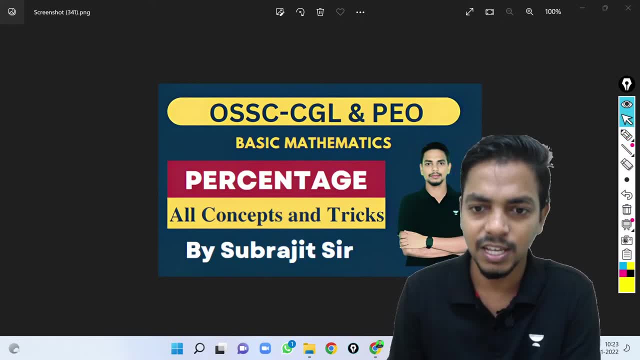 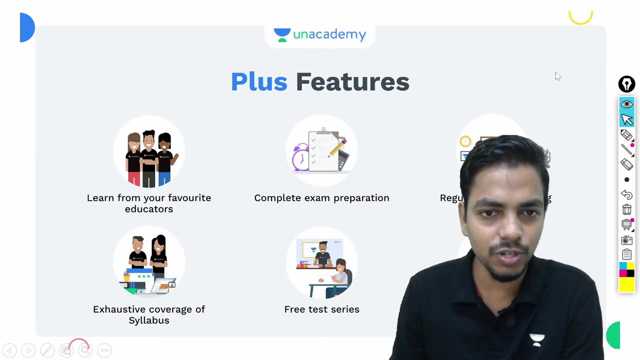 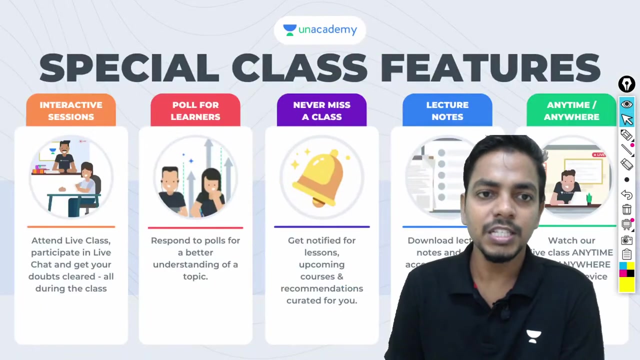 I will tell you what percentage it is. I will tell you what percentage it is. If you don't have a plus subscription. you will get a very big offer and you will get a plus subscription very soon. You can also apply by book or email. 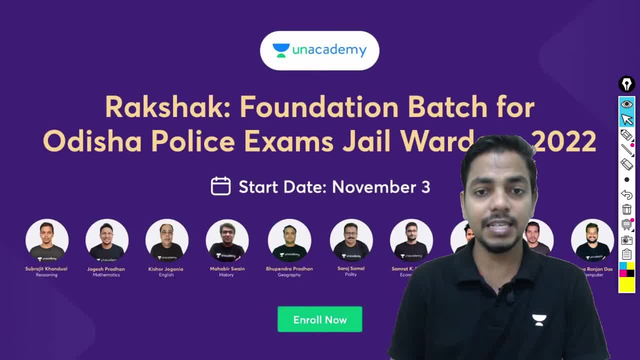 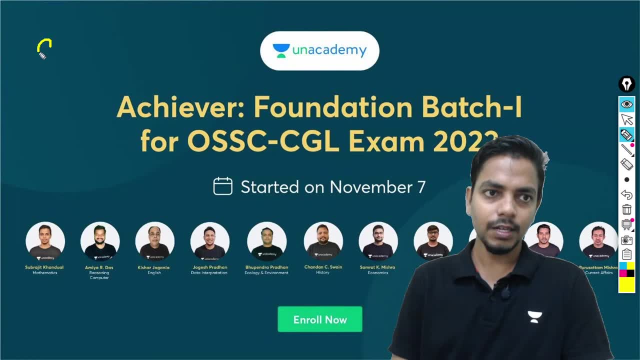 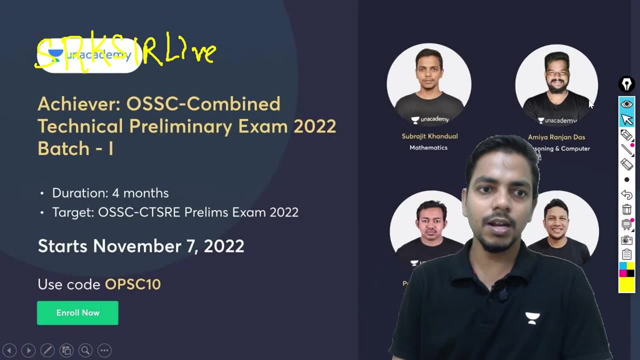 Many students are also waiting for exams. Be many, Be many, and please do not forget to subscribe. If you like this video, press the like button. Thank you, code srksrlive. use the code and get the plus subscription as soon as possible. yes, cjl. 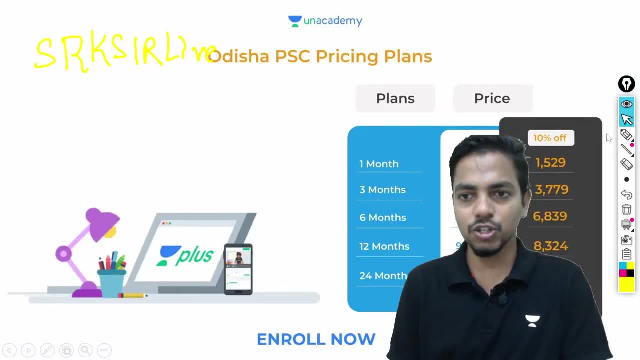 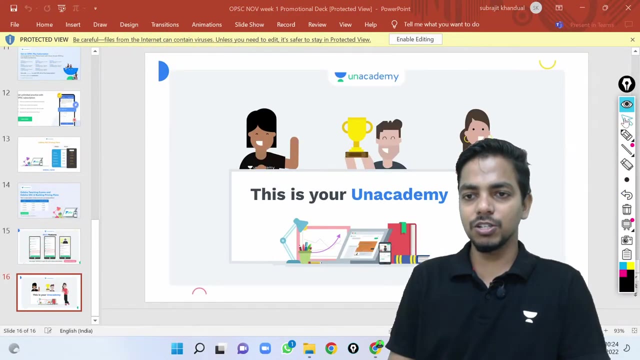 lobby has also started the class today. the PEO has also started. we know the price structure. if we use a referral code- srksrlive- you will get the maximum discount. yes, let's start today's session. yes, let's start the session. I will tell you in advance. you can. 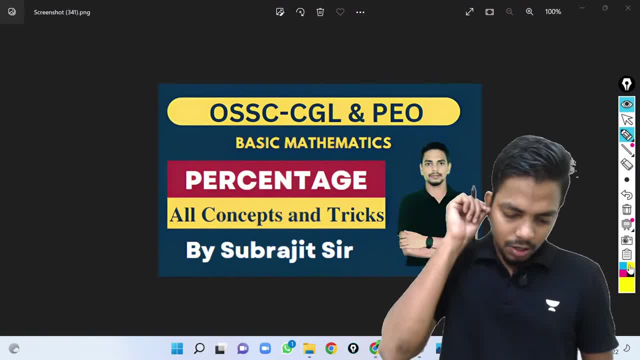 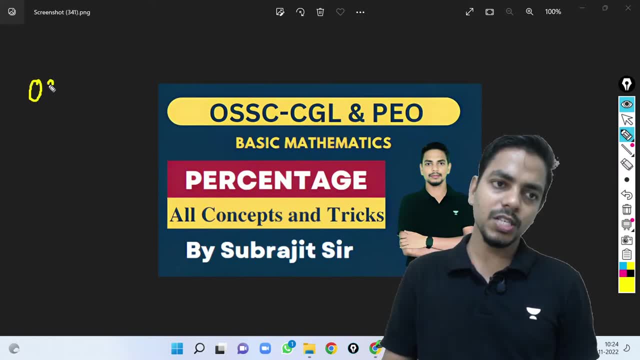 click on the session, all the sessions that we have started from the button. you will remember that these sessions are specially brought to the OSS CGL. I have not prepared a special session for PEO. if you get a center, get a CGL or get a MTS or get a CPO, get. 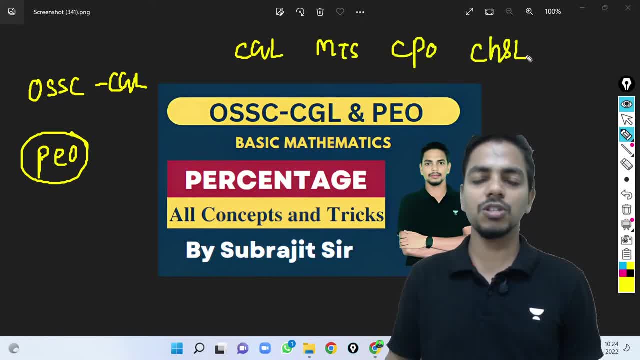 a CHSL. you will be very useful in these sessions. well, you knew it would be mostly free class. I will keep it. I will tell you in advance. they will tell you to get training. they will also inform you. I will not give you any kind of reason. I will explain to you. I repeat. 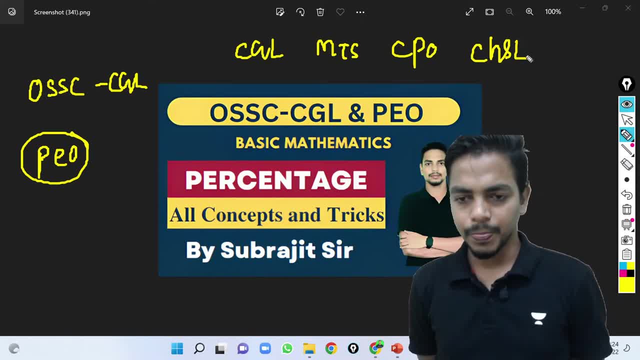 it to you. I have to give you an example. but first there will be nothing to do. I will. I will provide you free material, Whether your Mathematics, English Reasoning, GS, Whatever message you have sent me, I have already received it. 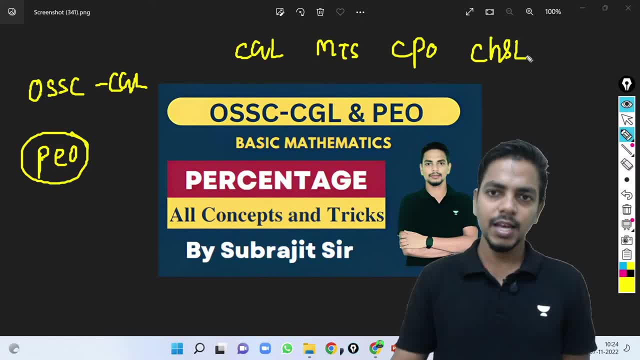 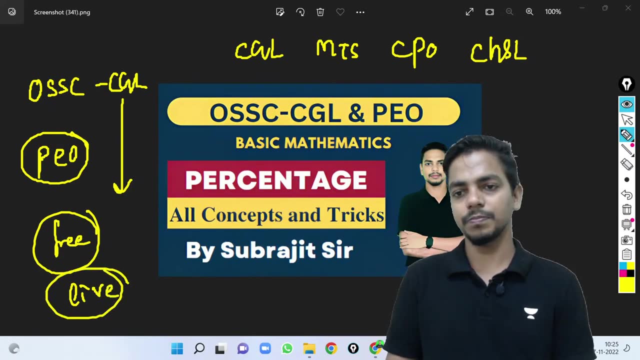 If you have not received it, I will send it to you. I will give it to you for free. there is no payment. I will give you the complete syllabus for free. I will send you the material. I will send it to you for free. I will try to bring you to the class. 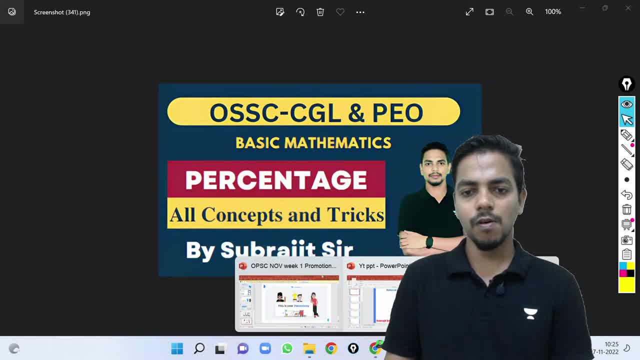 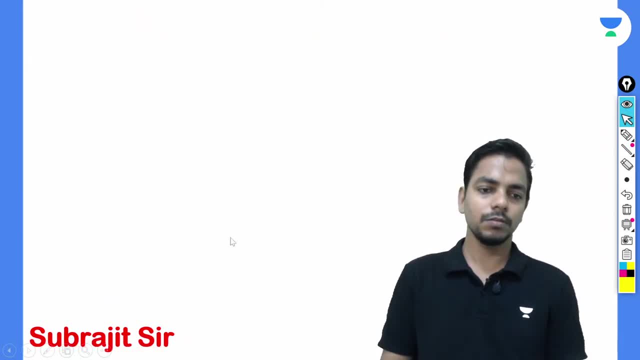 I will present the full teaching. I will put you through the course. I will put you in ohneology. You can share it See Hello, Heeding the Idea of Percentage: Write down, guys, I will 배. If you don't write it down, it doesn't stop. 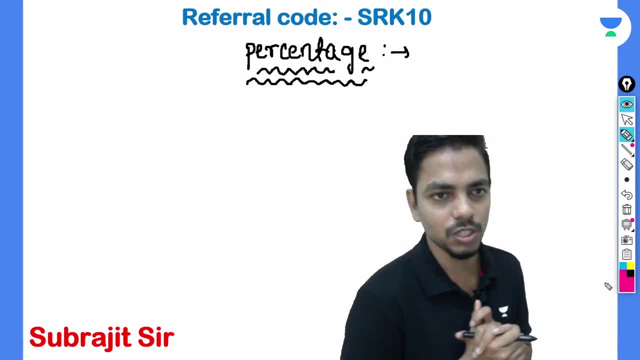 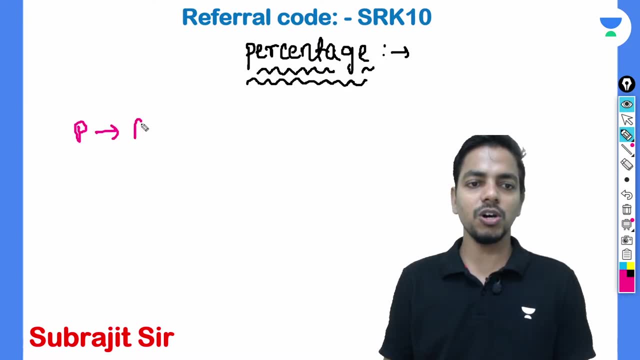 As I told you earlier, your love calculator is here. Which love calculator? Pratyushahita Anjali? Who is here? Pratyushahita Anjali, you are getting 98% love. Or if I say: 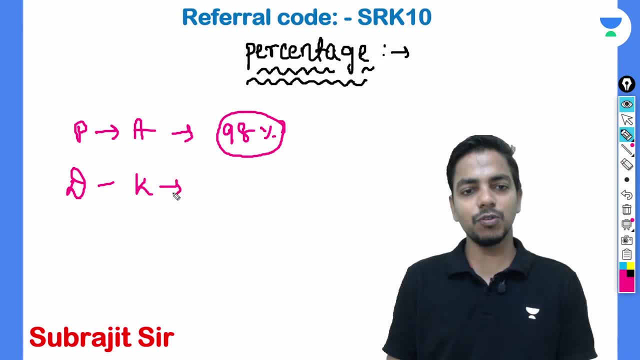 Devashishahita Kaveri, you are getting 38% love. If you had used love calculator earlier, you would have got 98% love. Why is that? If you are going to take exam, you are getting 45% love. 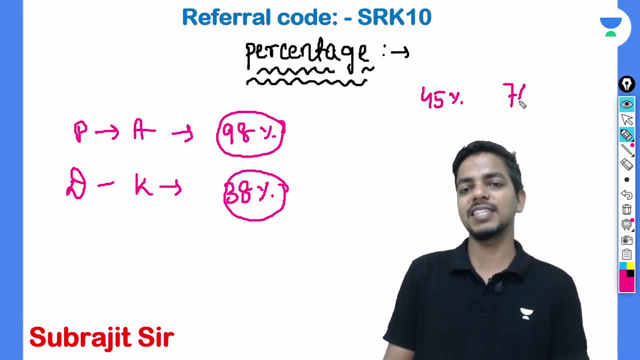 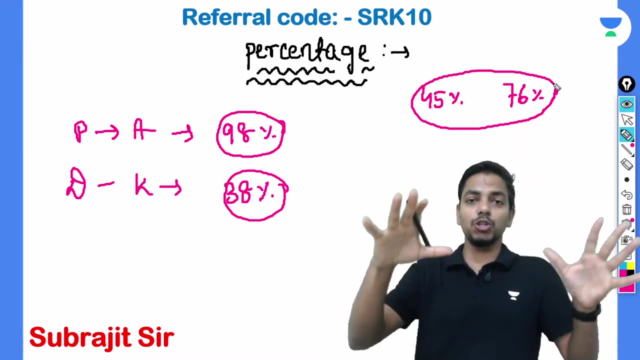 If you are going to take 10th exam, you are getting 76% love. This is what I am getting. If I say Pratyushahita Anjali, I am getting 98% love. Pratyushahita Anjali. 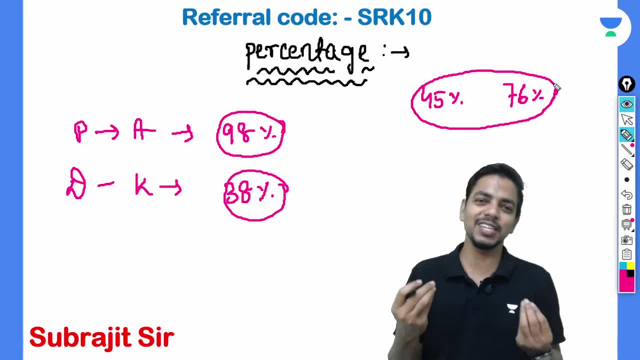 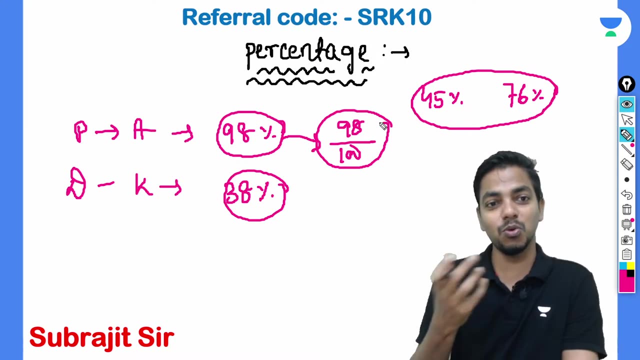 you are getting very happy. You are saying: my father loves me so much. I am telling you This: 98% love. if I write, you will get 98% love. If I had used love calculator earlier, I would have got 98% love. 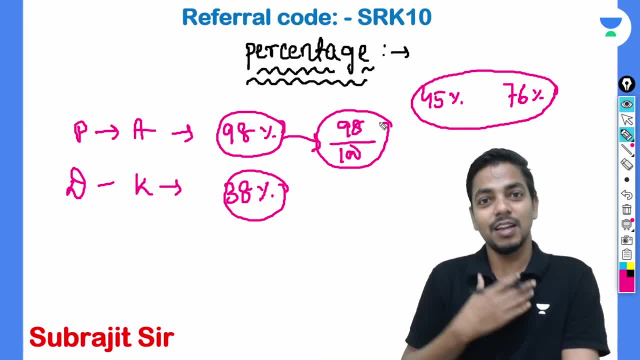 Pratyushahita Anjali, you are getting 38% love. If I say Devashishahita Kaveri, you are getting 38% love. 38% means 38 divided by 100.. That means 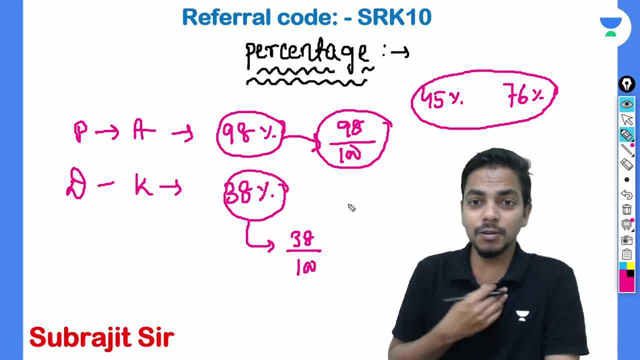 you are getting 36% love. That is it. If you had kept 10th exam, you would have got 32% love. I am telling you: 32 out of 100.. 36% love, 76% means. 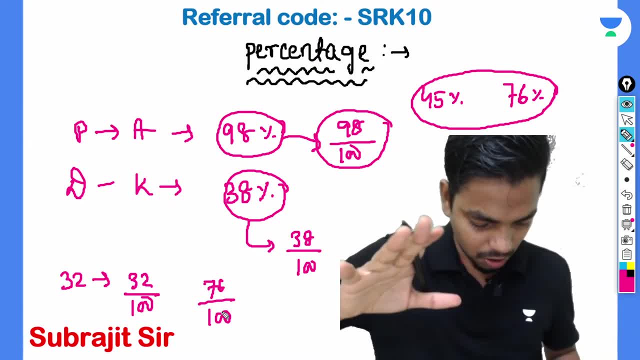 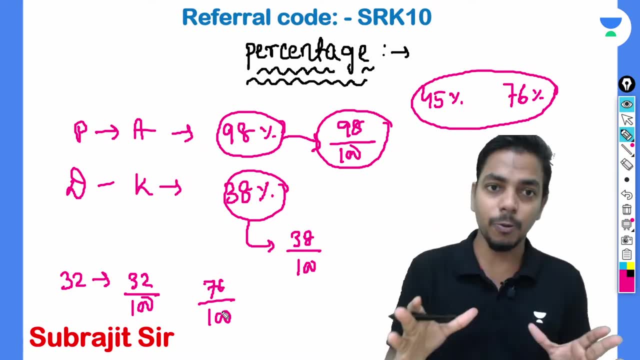 you are getting 76% love. That is it, Whatever I had written, whatever I had written, you have to read it freely. Read it freely. You have to take the subscription or not. that depends on you. If you have not taken the subscription, 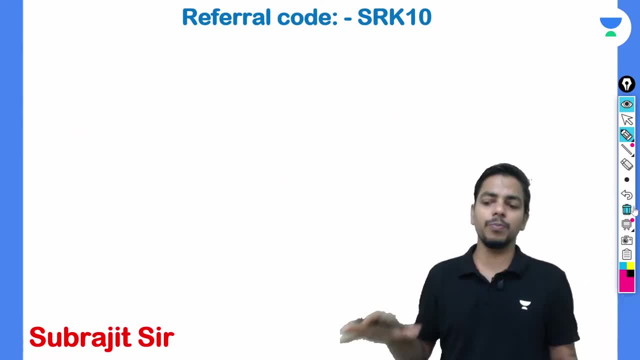 you have to use the referral. The second thing: you have to complete the entire syllabus. if you have not taken the BAT, Just do it freely. If you have not taken the class link, you will have to message me. So 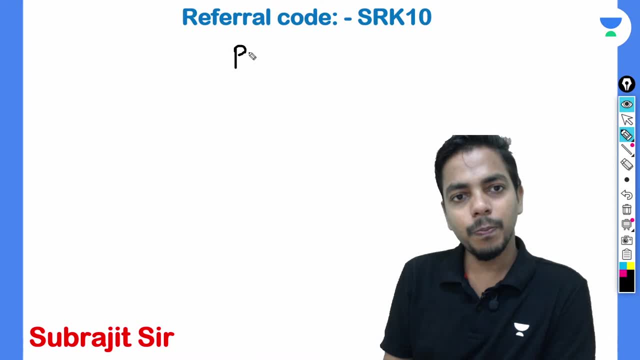 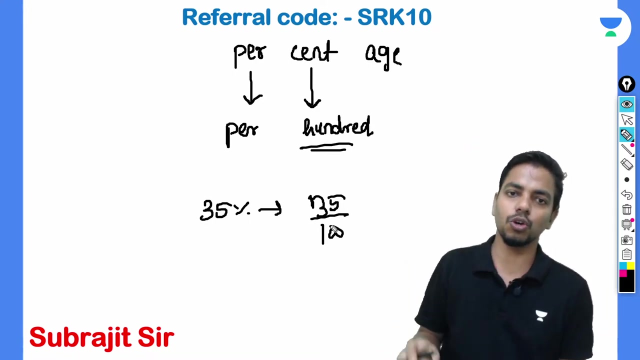 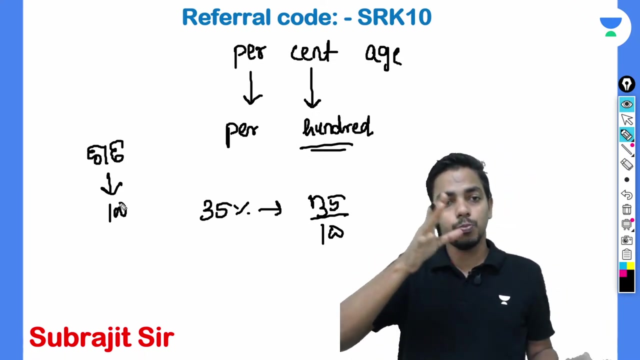 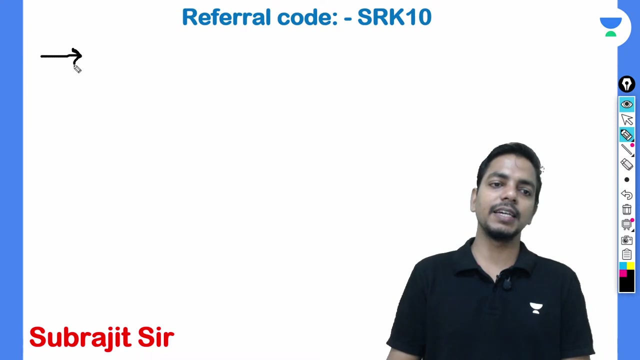 you need to know the percentage. cent is per means. every cent means 100. how much is every cent? if I say 35%, then every cent is 35. each hundred means every cent. there is no place to put percentage. taken it. well, OK, So if you write the first heading is a part out of 100, or you can say percentage is a. 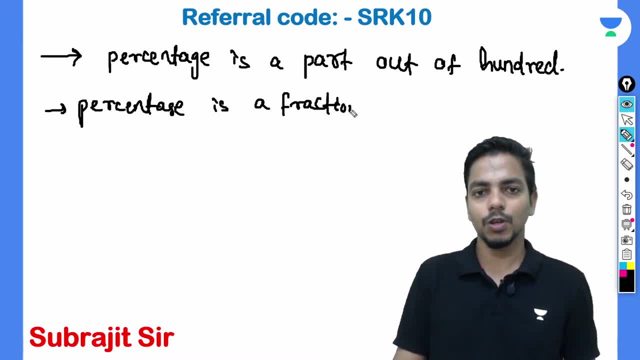 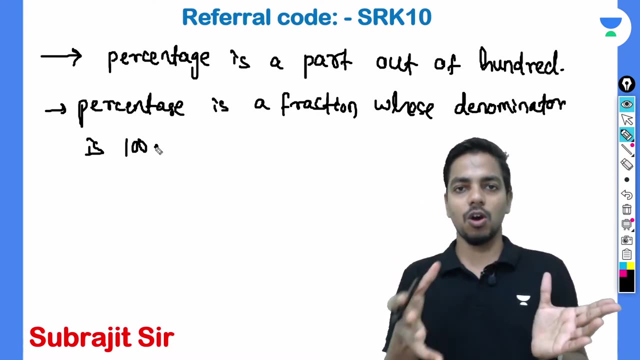 fraction whose denominator is 100.. Percentage is a fraction. What is a fraction? It is a fraction of some part. It is not a fraction but a part. It is not a part of a person, but a part of a person. My friends, I am telling you that there are 500 parts in a person. 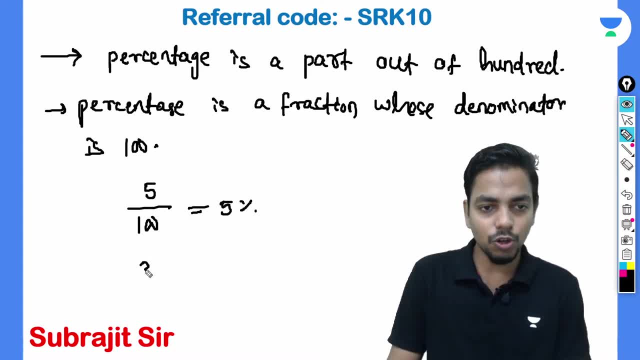 You will say that there are 500 parts in a person. I am telling you that there are 500 parts in the person. So I am telling you that there are 500 parts in a person. All of them are the same, So it is a fraction of 100.. 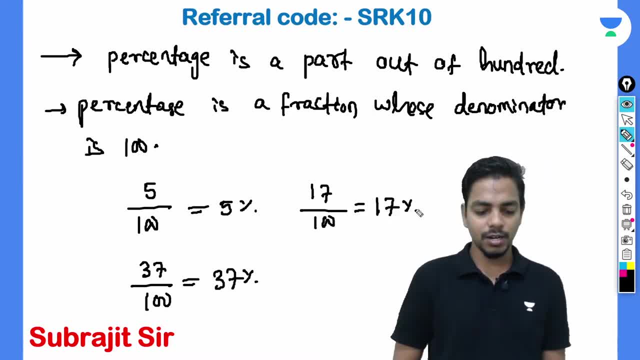 So if you write the first one, you will say that it is a fraction of 100. there It is a fraction of 100, okay. So let's say that there are 500 parts in a person. Then we will say that it is a part of a person. part. 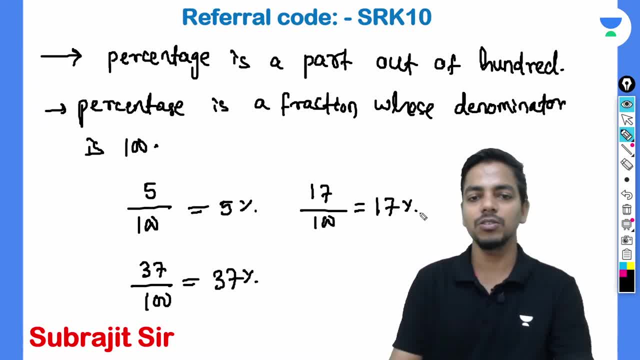 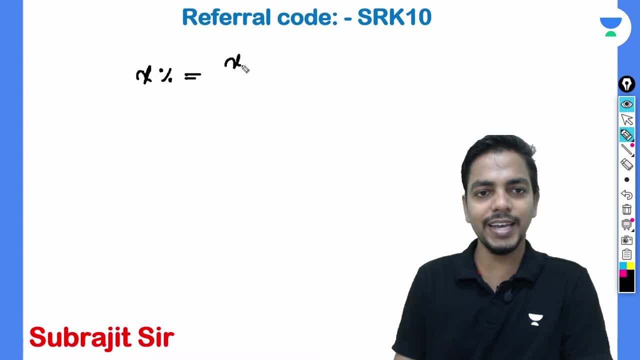 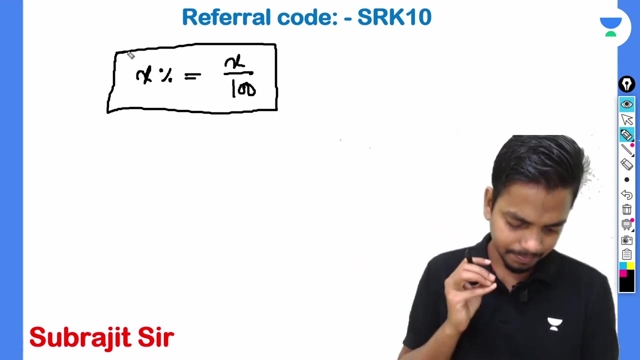 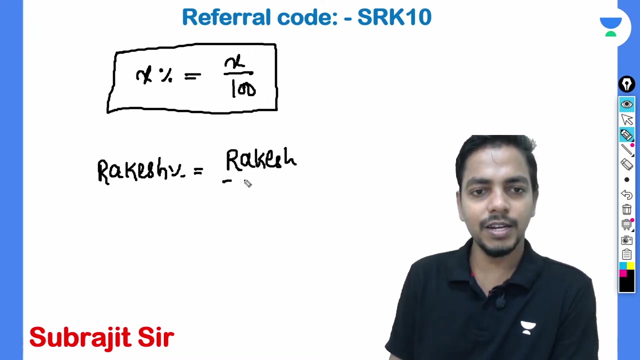 So write down the next part of the formula, that if I tell you X percent, I will tell you X divided by 100, which means that if I don't want it, it will be active in the class. If I tell you X percent, you will tell me: or X divided by 100. 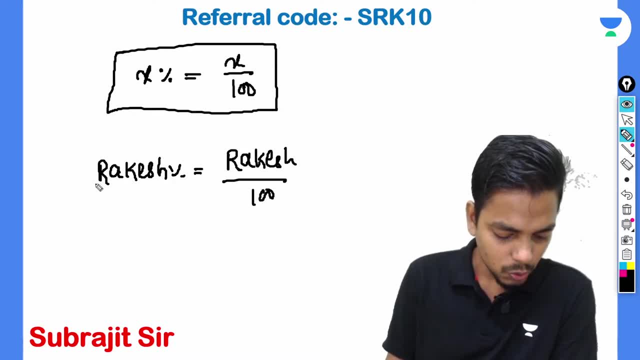 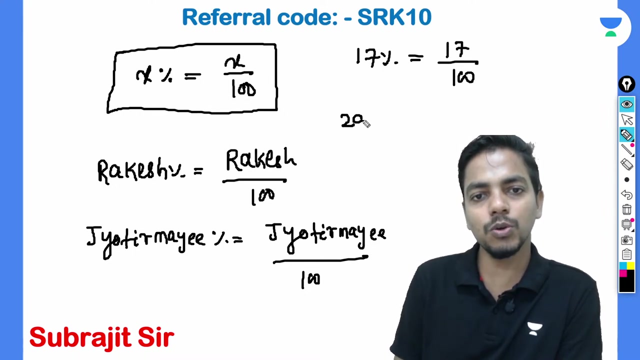 If I tell you X percent, you will tell me: or X divided by 100.. What did I say? 17% divided by 100.. If I say 17%, you will say 17 divided by 100.. If I say 29%, you will say 29 divided by 100. 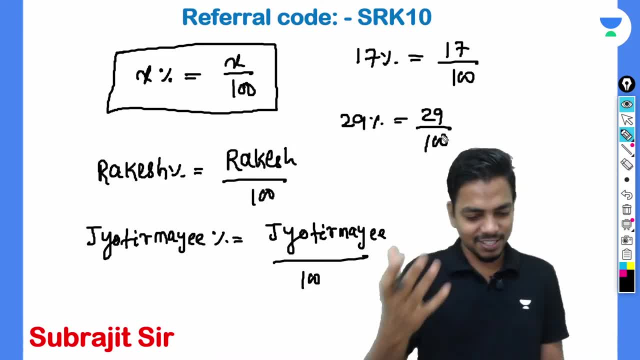 Did you write it? Yes, This is called pure SRK. Pratyush Das himself is commenting: Sir, you don't write, I will write: Pratyush percent is equal to Pratyush divided by 100.. What a thing. 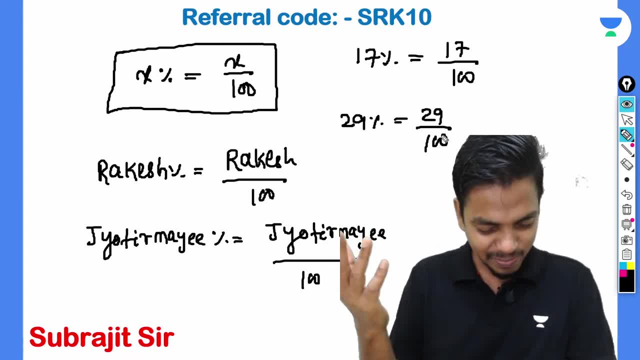 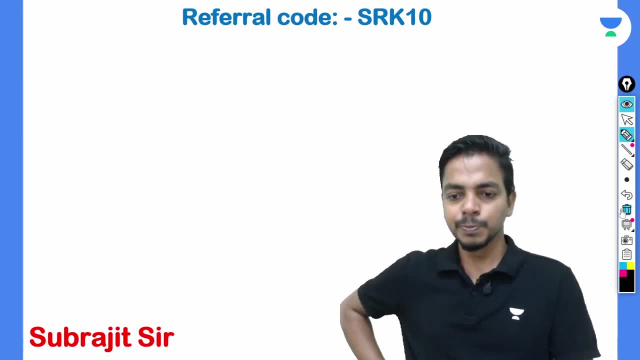 You have brought so much energy. Subrajit, sir, percent Subrajit divided by 100.. Wow, Thank you so much. God bless you. Come on, You will know the first formula. It is equal to X divided by 100.. 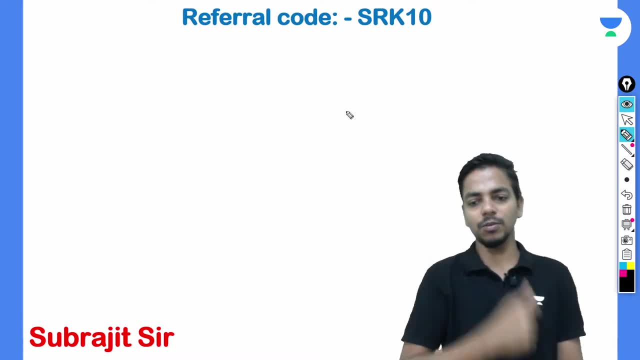 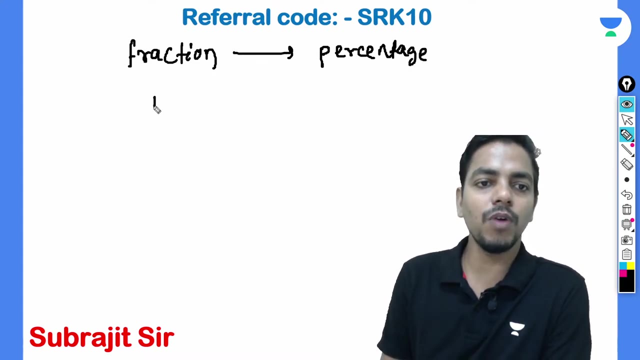 Do you know the second formula, Sir? which is the second formula that I am telling you? No, It is fraction. The time you will convert by percentage, Which will you do? No, I will say 1 upon 2.. The time you will convert by percentage. 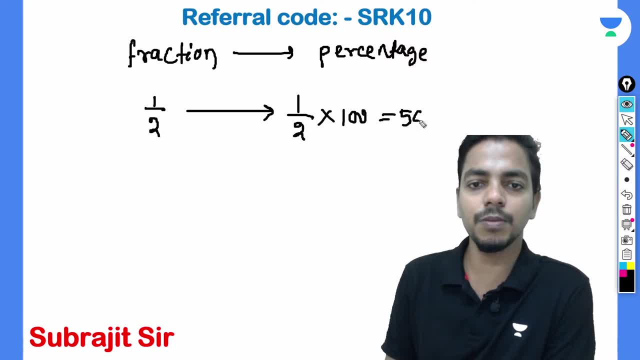 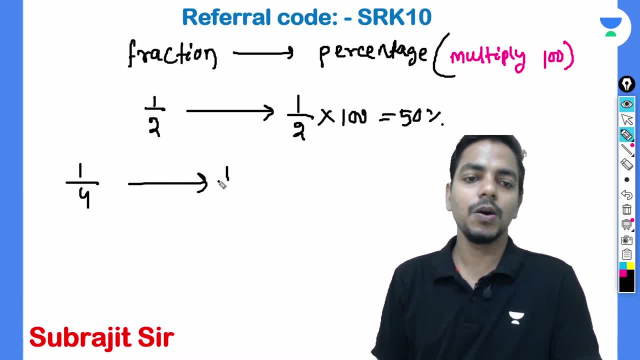 I will say 1 upon 4.. You will say 1 upon 4 into 100. Which will be 50%. I will say 1 upon 8.. You will say Okay, I will say 3 upon 4.. 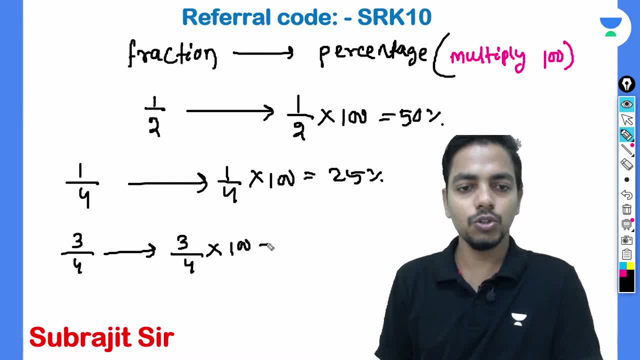 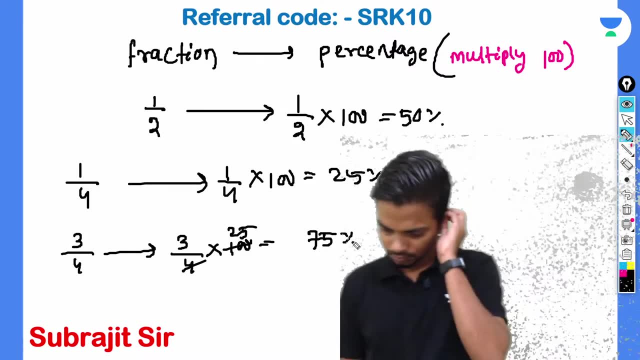 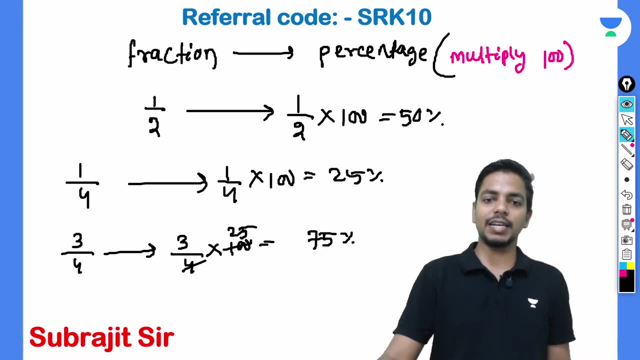 You will say 3 upon 4 into 100., Which will be 4 divided by 25.. 25 percent. I will say 3 upon 4 into 100. Which will be 4 divided by 25.. 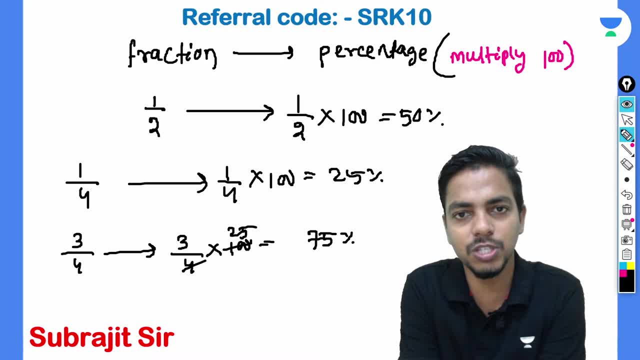 25 percent, I will say 3 upon 4 into 100.. Which will be 4 divided by 25.. 25 percent, You will say 5 into 100.. 50 percent: 5 into 100.. 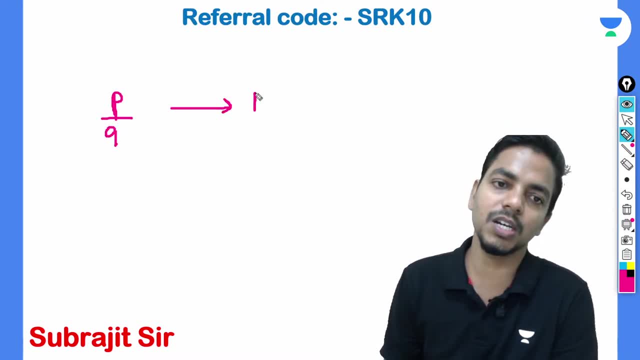 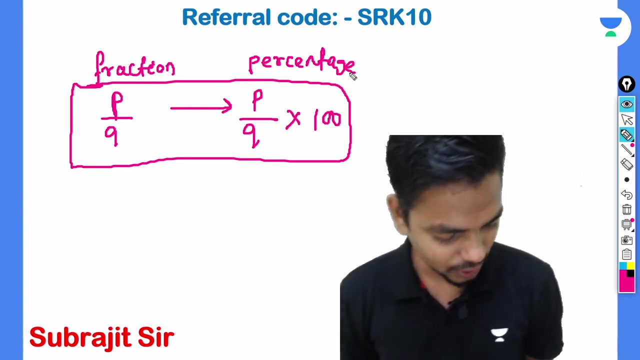 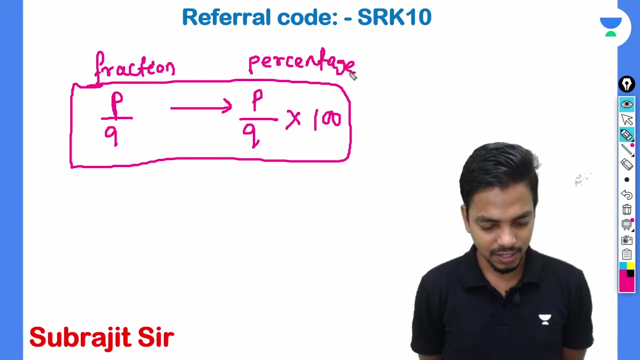 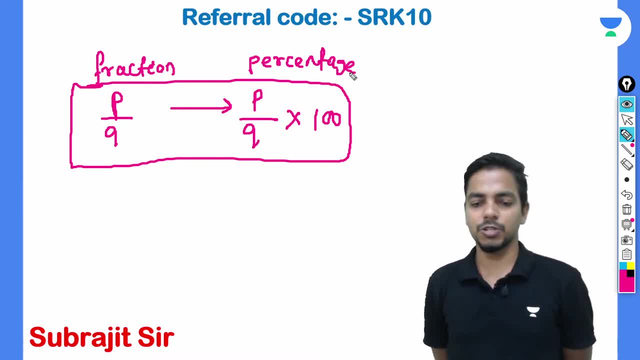 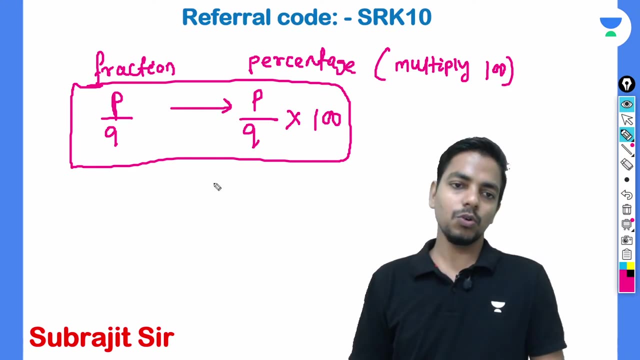 So what percentage of fraction did you convert or count? What did you write on the side Multiply? Did you get it? Is there any problem? Do you have a total series? What do you think? If you have a total series, you will get CGL and PO. 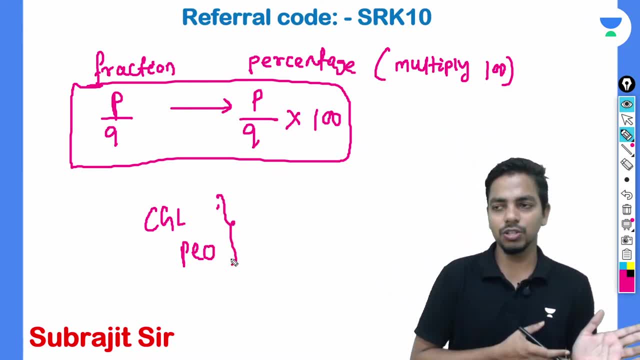 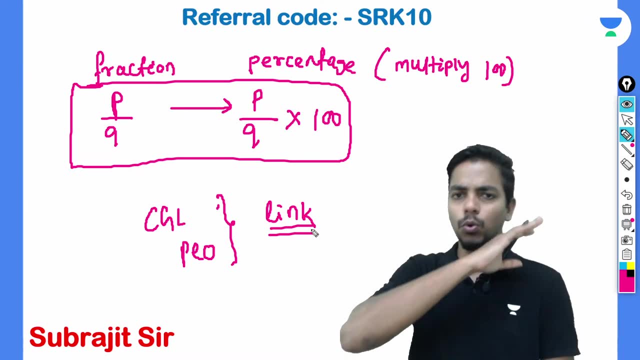 Before the total series. we have already mentioned that we need a link to a Korean class. I will send a message to the number system. I will send a message. I will send it for free. You will get no payment for this. I will write comments and will send it to the number system in the place where you are sitting, where you are doing the class. 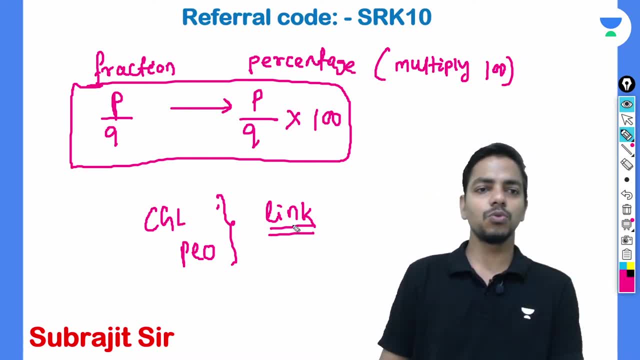 I will write comments and will send it to the number system in the place where you are sitting, where you are doing the class: Instagram, Facebook, YouTube- by searching any company, you will find Subrajit sir. I will send a message to Subrajit sir and he will give you free PDF material, class and link. 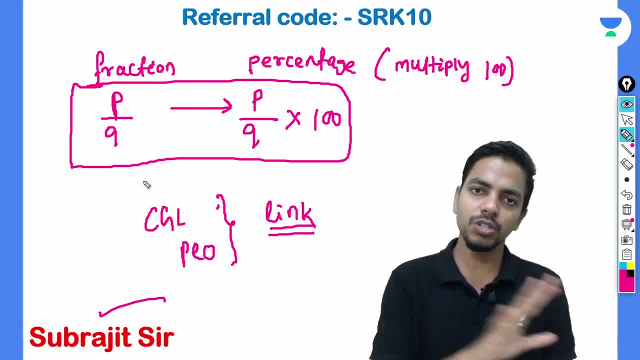 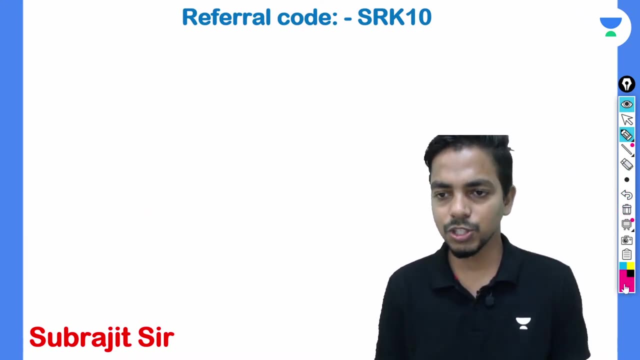 Everything is free. No check, no condition. You will message and you will get the materials. You will get free material, class and league. Let's see how to convert fraction to percentage. Let's take an example. If I tell you to convert percentage to fraction, 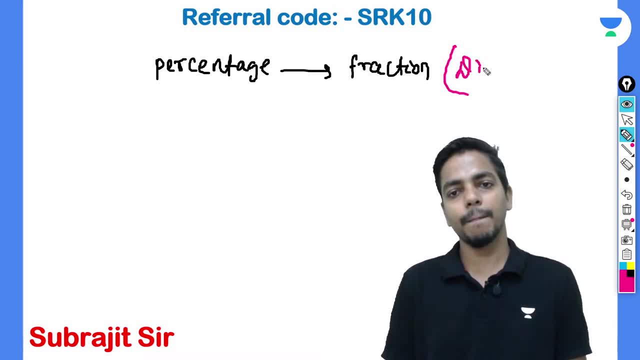 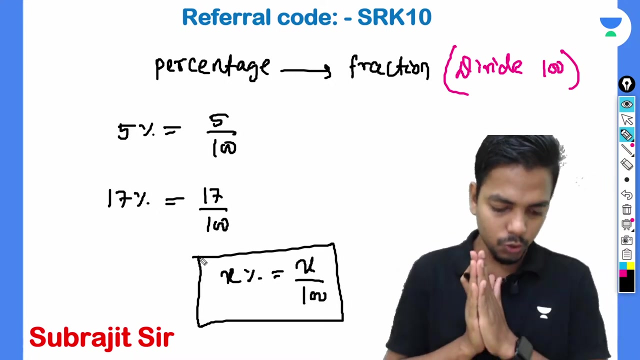 Write it on the side. Let's take an example: 5%, 17%. Write the formula: x% will be equal to x divided by 3.. If I keep the formula in the box, you keep the formula in the box. 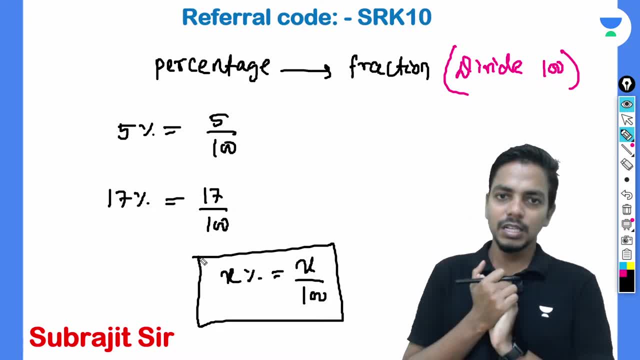 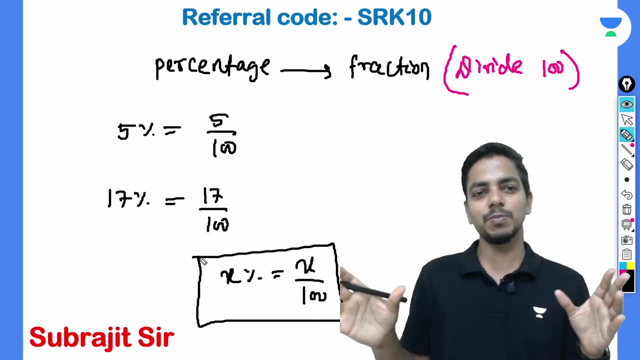 Otherwise it is a hospital. You will get the photo, Take a screenshot and edit it in the application. The whole of Chris Gayle was covered by the color of Steven Smith. Do not worry, You can also clean it by washing it with soap and rubbing it. 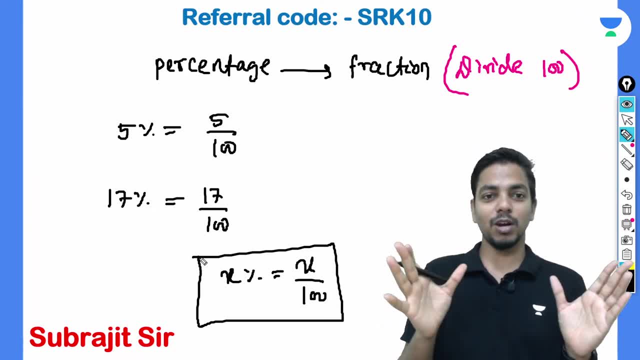 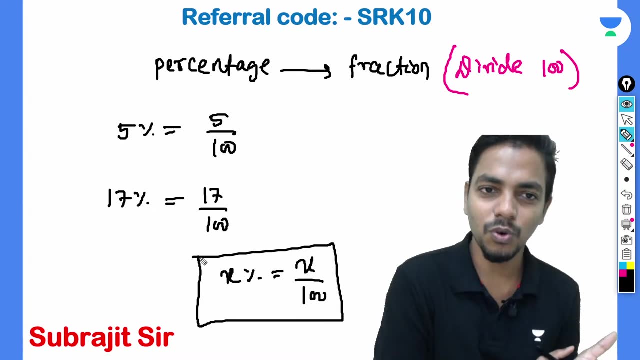 Only the photo. If you are in love with mathematics, you will have to learn it. you will have to keep the formula. you will have to keep the formula. you will have to keep the formula. the more you practice, the better your mathematics will be. 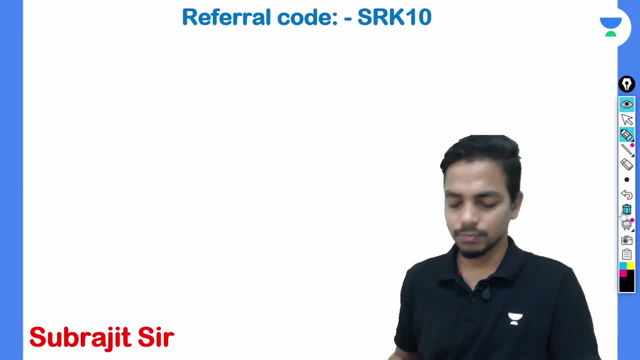 Okay, let's move on to the next part. There are some doubts in the writing. Look at the present. Let's talk about something else. Let's say: every day, Every day is a day, If in the calculator, in the calculator. 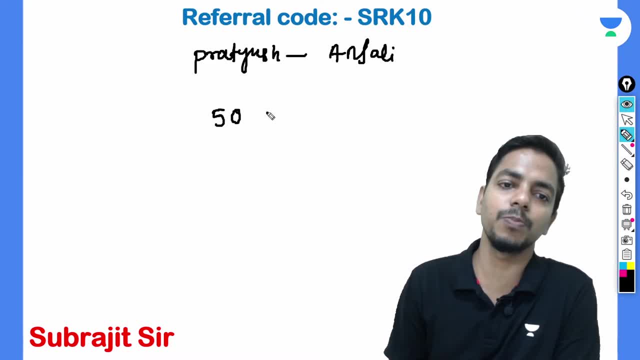 in the calculation she got 50% of her love. How much does that mean? If she got 50% of her love, then you can say that all 50% of Anjali's heart has 50% of love. 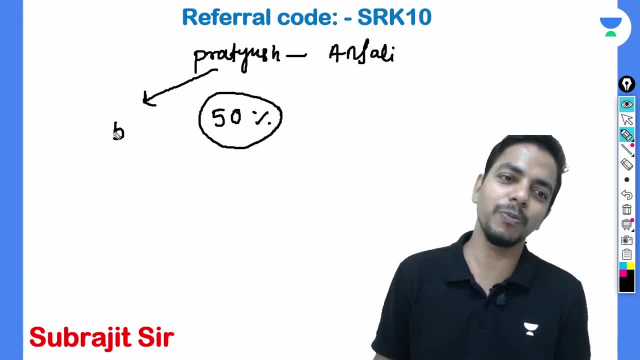 It means that 50% of her heart can be love to someone else in the future as well, Isn't it? Isn't it, Oh boy? So 50% means that 2 people are equal to 100,. this is what you will say. 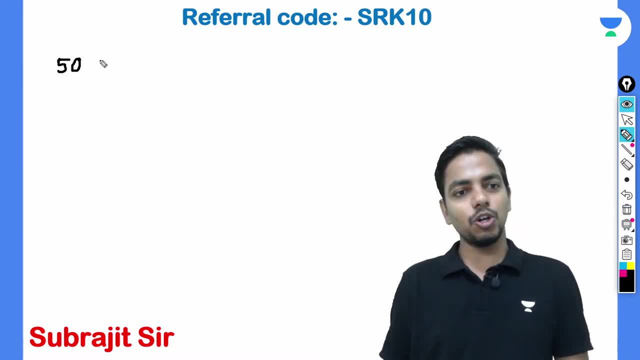 So you are saying that 50% is equal to 1 upon 2.. 1 upon 2 means that 2 people are equal to 100. So you can convert fraction into percentage. If I say 1 upon 2, it means 50%. 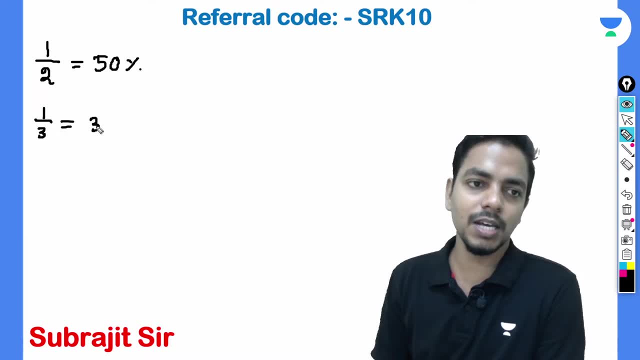 If I say 1 upon 3, it means 33 whole 1 upon 3%. If I say 1 upon 4, it means that 4 people are equal to 100.. How many people are equal to 100?? 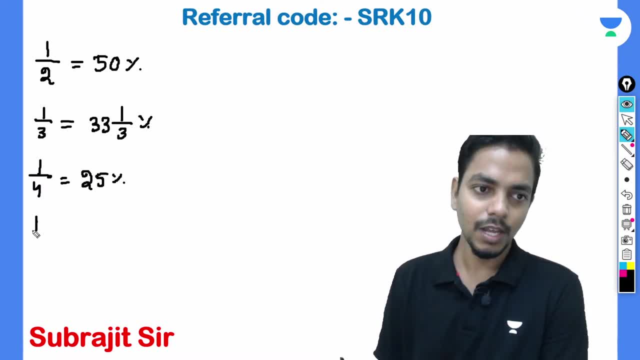 25% is equal to 100.. 1 upon 5 is equal to 20%. 1 upon 7 is equal to 100.. 1 upon 6 is equal to 16 whole 2 upon 3%. If I say 1 upon 7, it means that 14 whole 2 upon 7%. 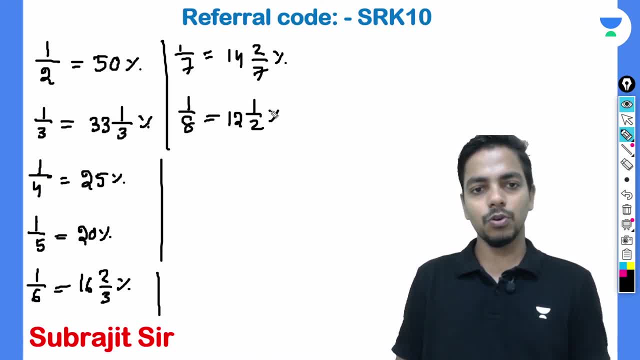 If I say 1 upon 8,, it means that 12 whole 1 upon 2%. If I say 1 upon 9,, it means that 11 whole 1 upon 9%. If I say 1 upon 10,, it means that 10%. 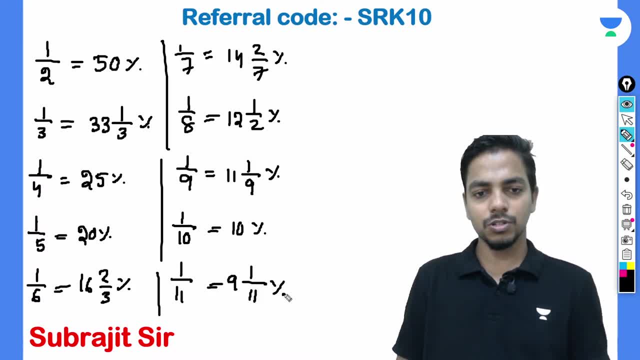 If I say 1 upon 11,, it means that 9 whole 1 upon 11%. If I say 1 upon 12,, it means that 8 whole 1 upon 3%. If I say 1 upon 13,, it means that 9 whole, 13 whole, is equal to 7 whole, 9 upon 13%. 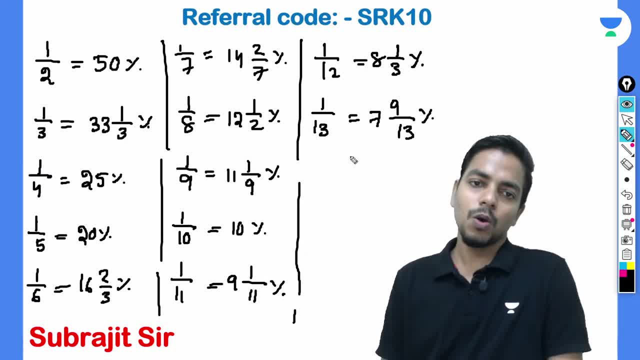 13 whole is equal to 6 whole. 9 whole is equal to 3 whole, 4 whole, 7 whole, 5 whole. What does 5 whole mean? 6 whole, 6 whole, 7 whole. 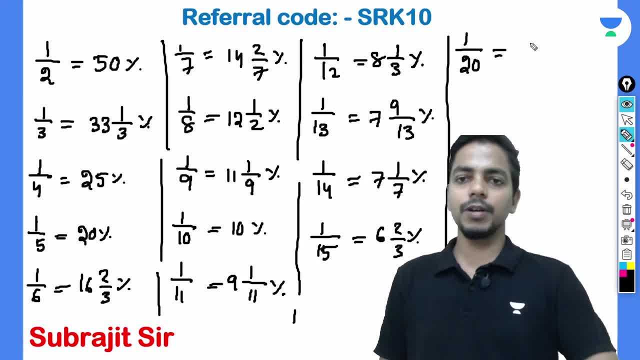 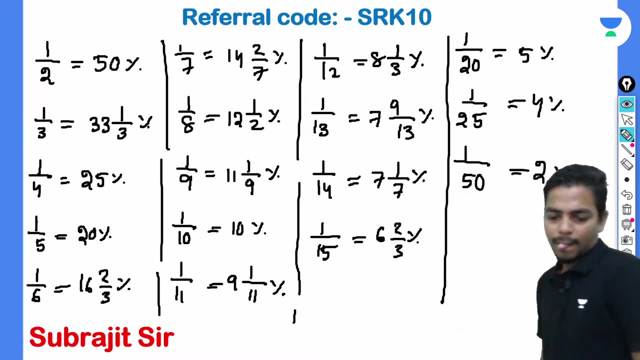 6 whole, 7 whole. 1 upon 20 means you will get 5%. 1 upon 25 means you will get 4%. 1 upon 50 means you will get 2%. write it quickly: 1 upon 16. 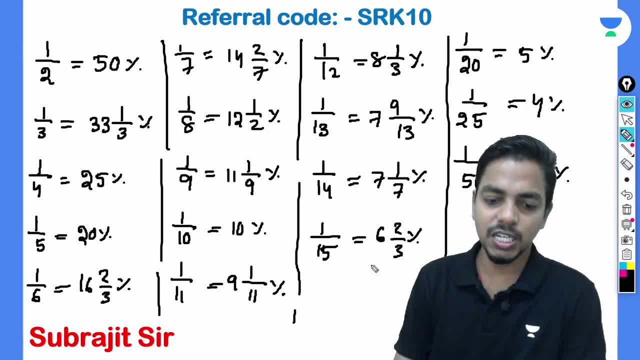 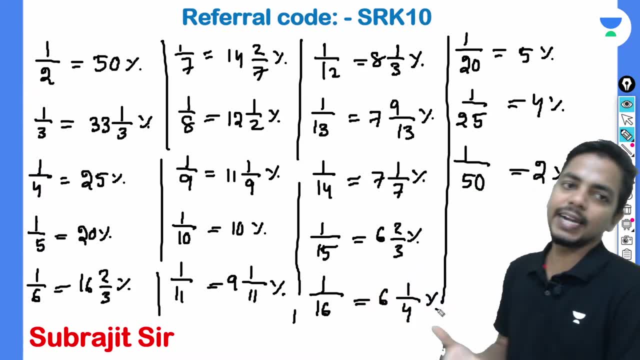 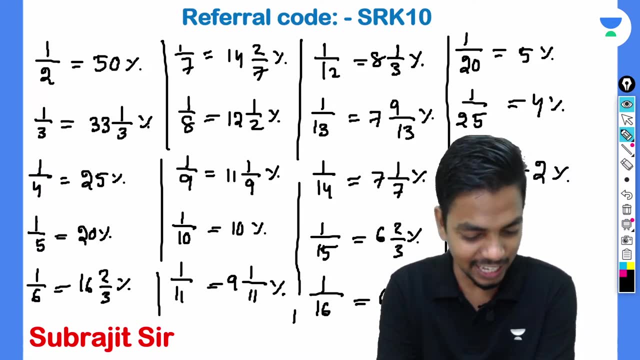 ok, you write it. 1 upon 16 means you will get 6%. if you have any idea, you can write it. I will tell you the whole thing. ok, see, today. today we are fighting. if you are in love calculator, if you are in love calculator. 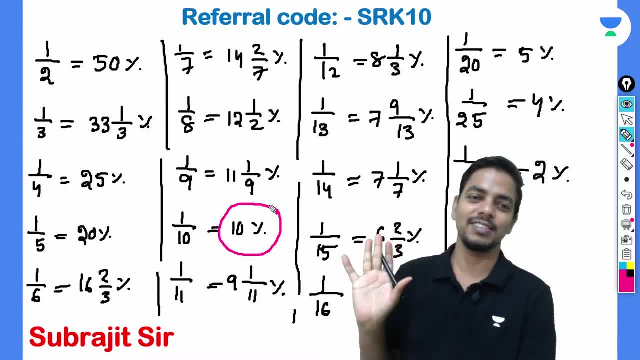 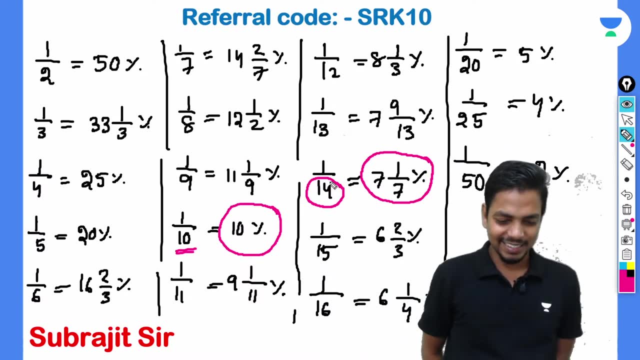 10% fight with each other. 10 people are sitting together. if you are in love calculator, 7%, 10 people are sitting together. what is the whole thing? 1 upon 7%, how many people were there? 14%, right, think, see today. 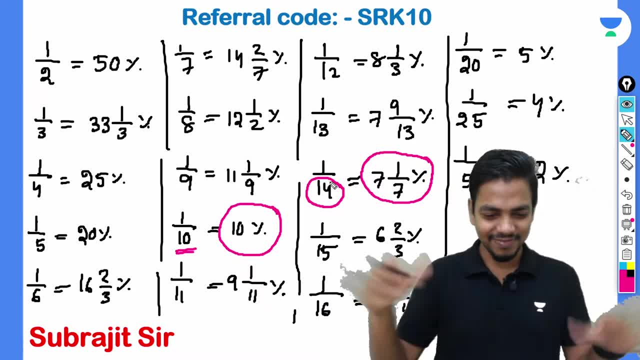 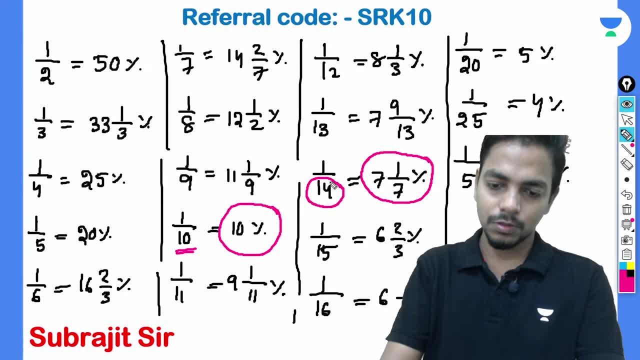 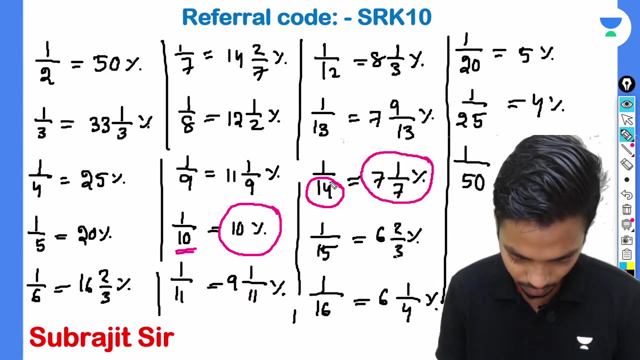 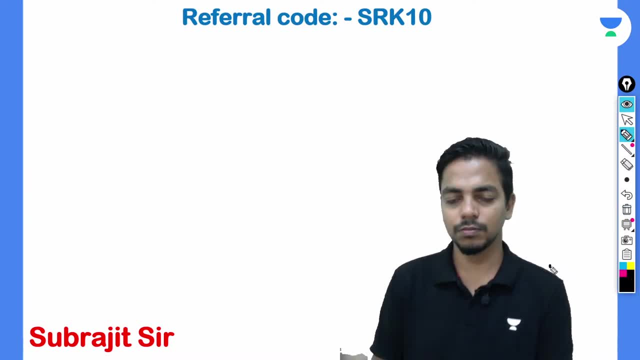 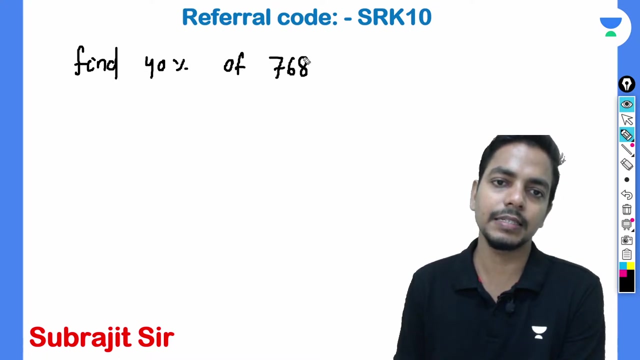 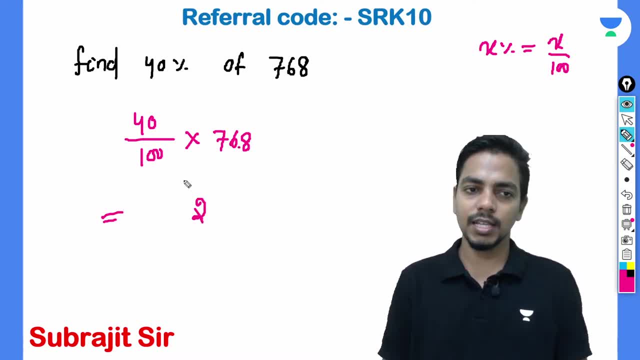 Multiply it: 8, 4, 32, 2, 3, 6, 4, 24, 3, 7, 4, 22, 7, 4, 28, 9, 3, 3, 3 Divided by 100, Which is 303.7.2. 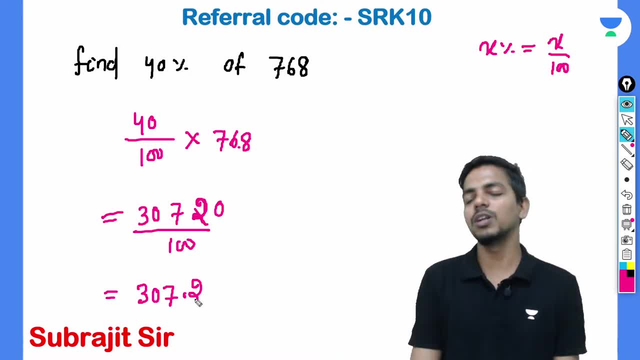 Do not do this every day. Do not do this every day. There is no problem if you do this every day. There is no benefit if you do this every day. CGL is very time consuming. It is time for March or April. 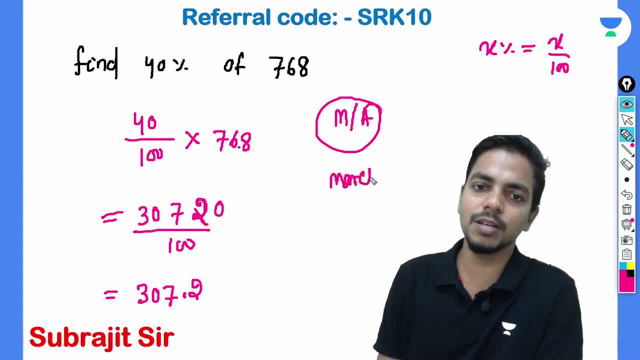 March or April exam can be done. It is not March If your exam is in February or March. See everyone had a mind. If you are doing this, See everyone had a mind. Give an example. Let's say I gave you a ball, Big ball. Let's say: I gave you a ball. 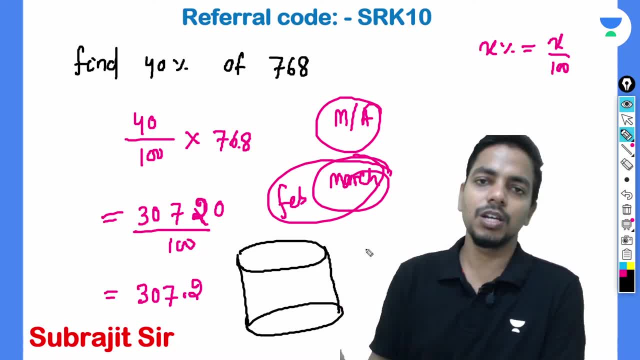 Let's say I gave you a ball. Let's say: I gave you a ball, Give me a ball Or you cut the ball. You can cut the ball in this way. Who will win? Start by cutting the ball on the first day. Maybe it will take 10-15 days to cut the ball. 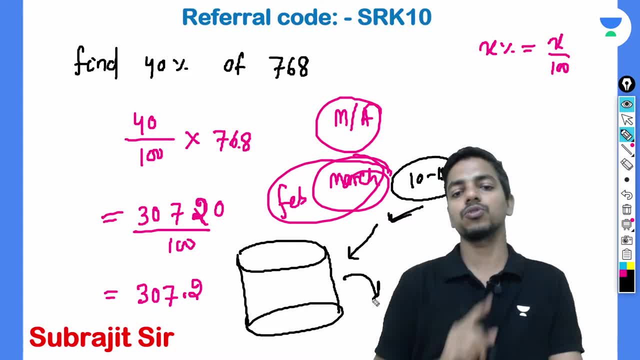 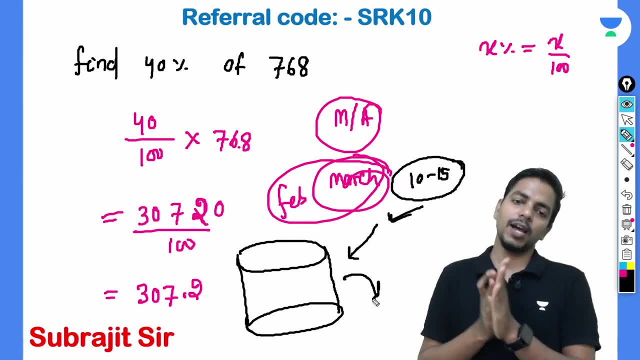 You will get the best chance. You will get the best options. See, You will get the ball and the ball Just because the ball is very big. You will get better. You will enjoy your school. Come to campus, See, you will be very happy. See, you will be very happy. 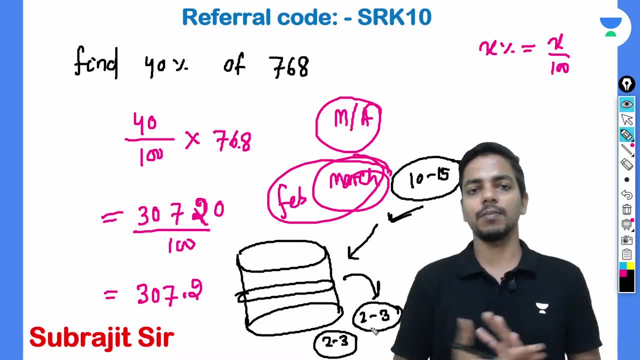 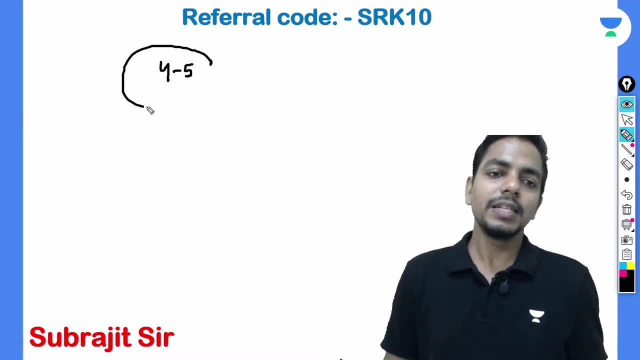 It will take you at least 15 days to complete the exam. I am not saying that it will take 4-5 months to complete the exam. It will take 4-5 months for you to clear the first base. We will learn the zero level and easy method. 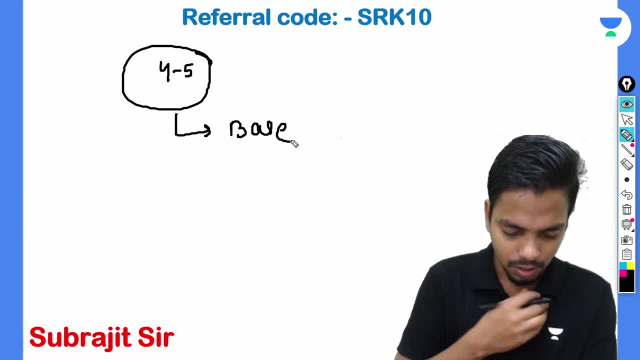 We will learn the basic mathematics. We will learn the basic mathematics and we will practice MCQs related to the exam. It will be a little difficult for us. For example, if you study in November and December, you will study the basics. 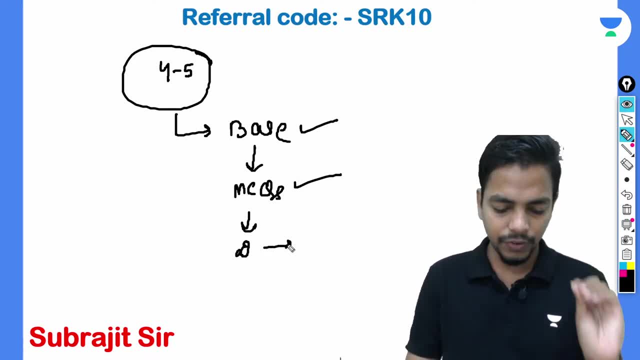 If you start MCQ in January, it will be a little difficult for you to complete the exam for a month. It will be a little difficult for us. If you study MCQs, you will face a lot of problems. Maybe your confidence will be down. 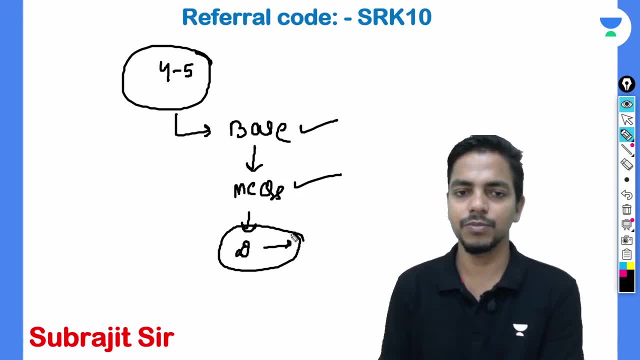 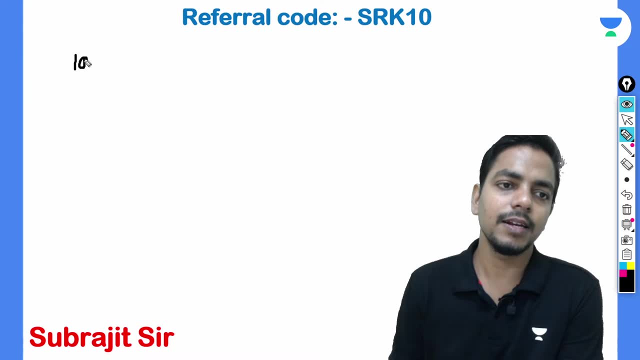 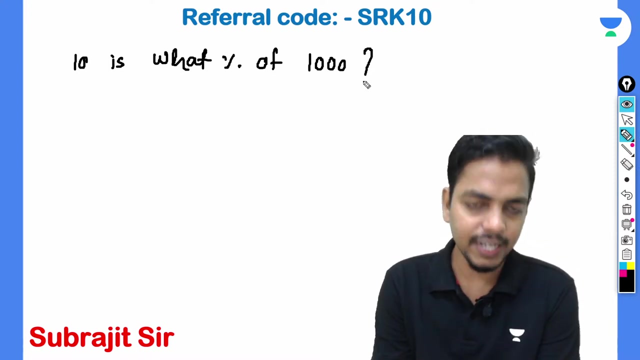 You will have a lot of problems. That's why it is called the basic level. Let's write another formula: What 10 is part percent of 1000.. Let's see this question. Rashmita Behera Pachachwanti. Sir will do a light class committee and will get a link committee. 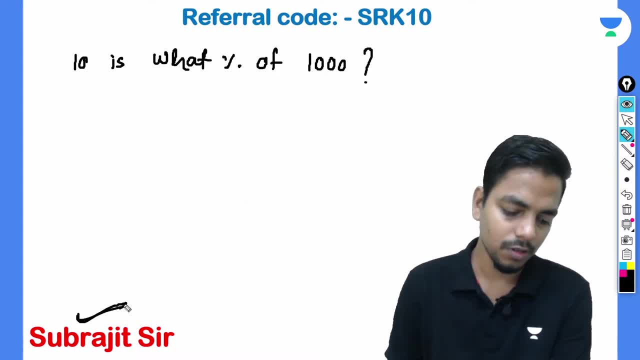 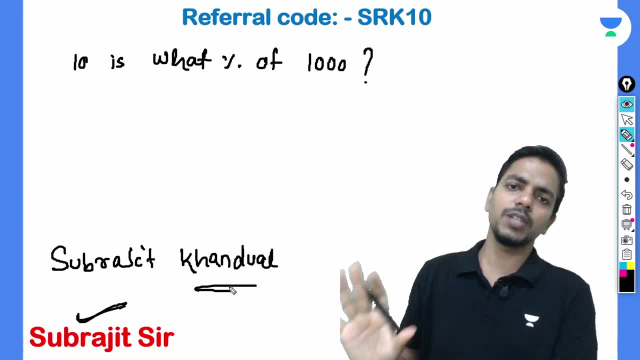 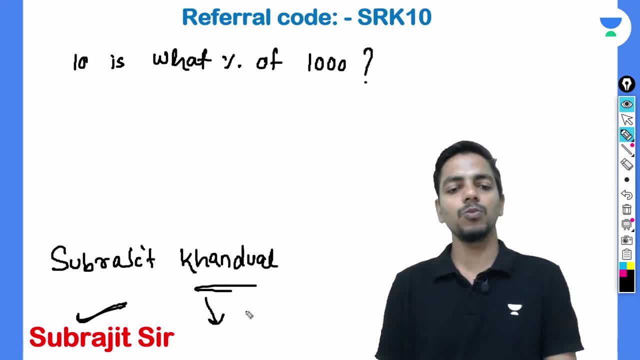 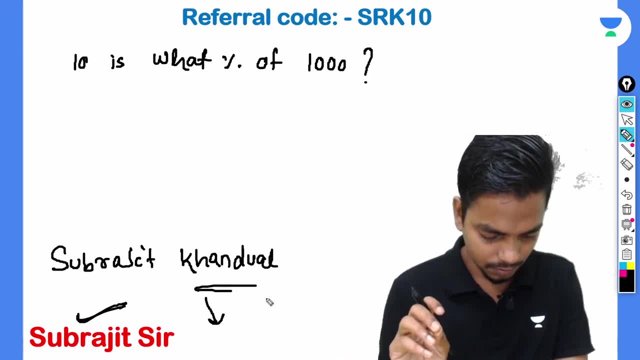 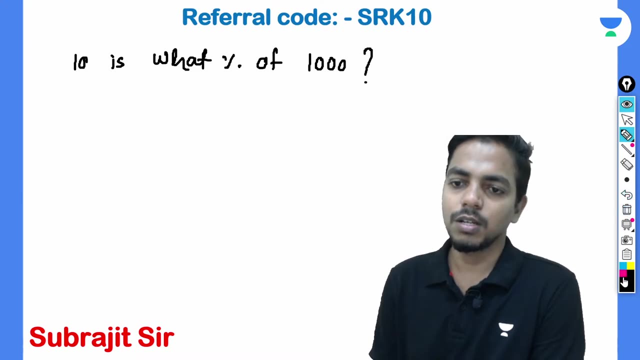 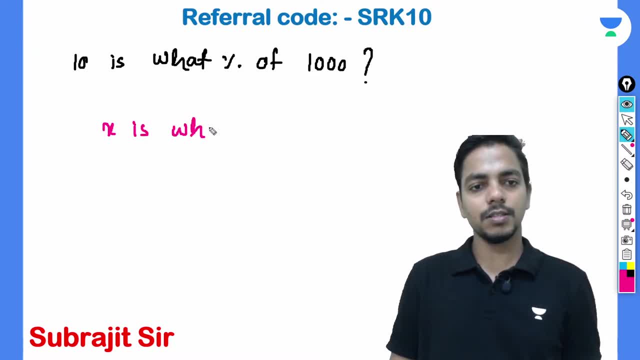 No, X is the fat percentage of Y. which formula do you want to use? No, I want to use the formula X upon Y into 100. See 10 is the fat percentage of 1000, which means X is the fat percentage of Y. 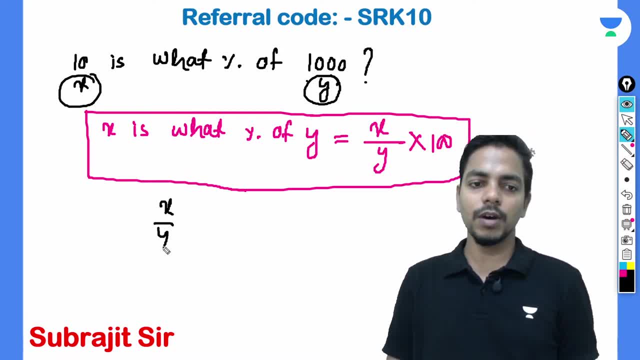 Which formula do you want to use? No X upon Y into 100, Which you can use. the value of X is 10 divided by 1000 into 100, Which means: listen to this, listen to that, listen to that, listen to that. 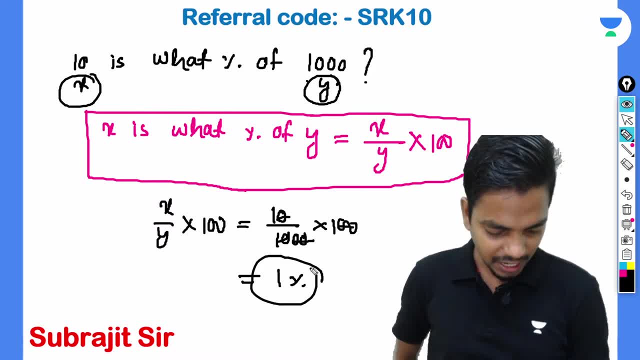 How much percentage do you want to use? 1%? What is this? It is the creation of the ocean. Thank you so much. God bless you. Participate right, It's fun. It's fun Class. Hello, You know, X is 40% of Y. That means X divided by Y is 200.. Box J means this is your formula. 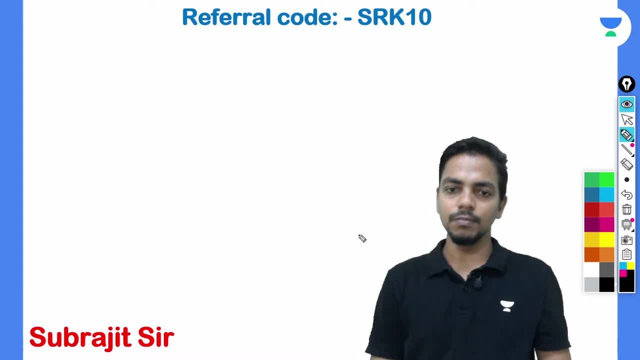 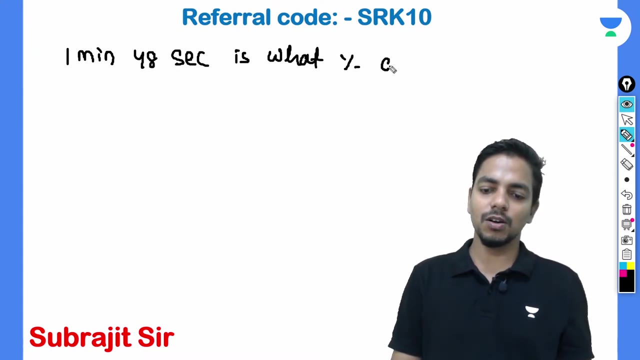 Let's move on to the next question. If I tell you, one minute 48 seconds is what percentage of one hour? Give me the answer to this question Now you have to write it down. Who is laughing, Who is angry? Who is angry? Let me know. 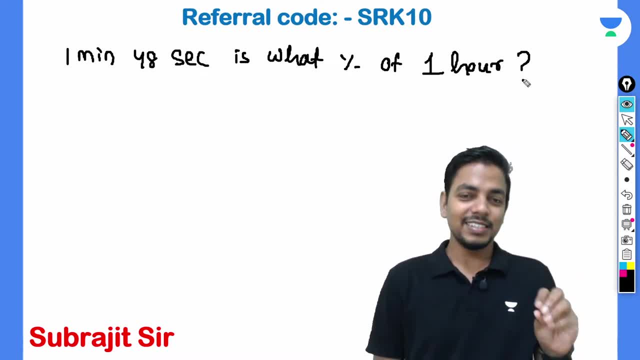 What is the answer? You are angry, Because you know you are angry, Don't you hear? Know that you are angry, angry, don't you hear. And if you keep thinking like that, that you are angry, angry, don't you hear. If you keep thinking like that, God, let the 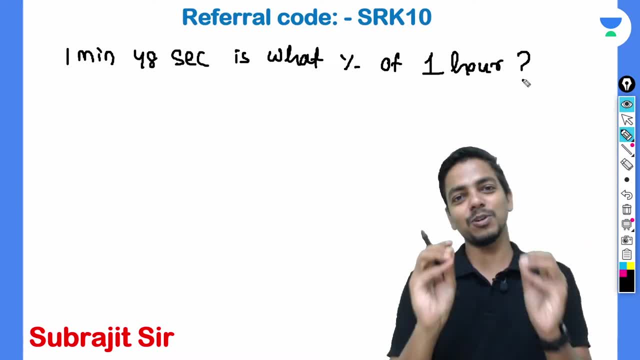 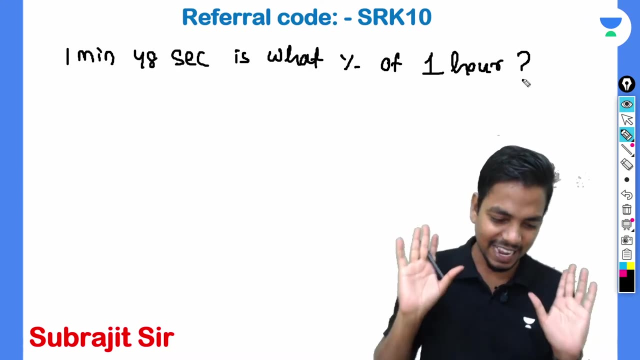 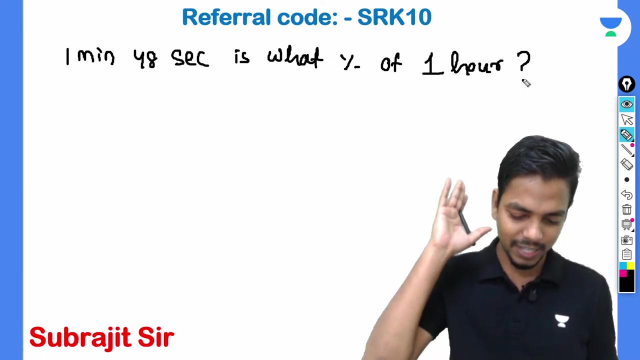 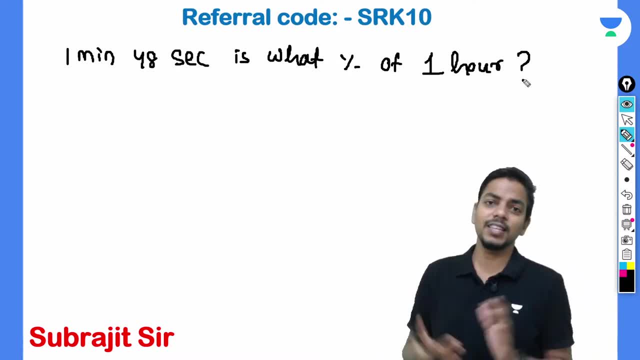 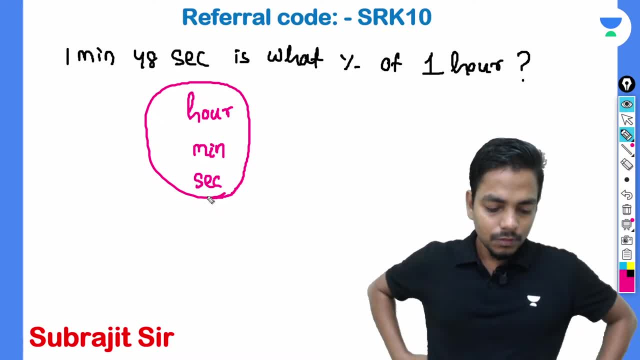 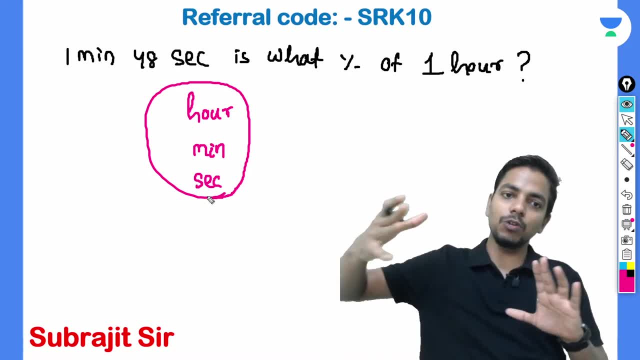 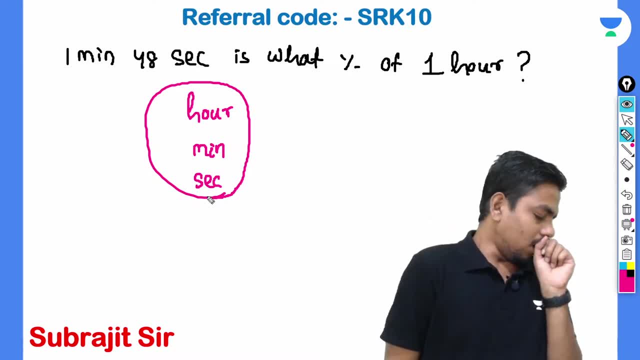 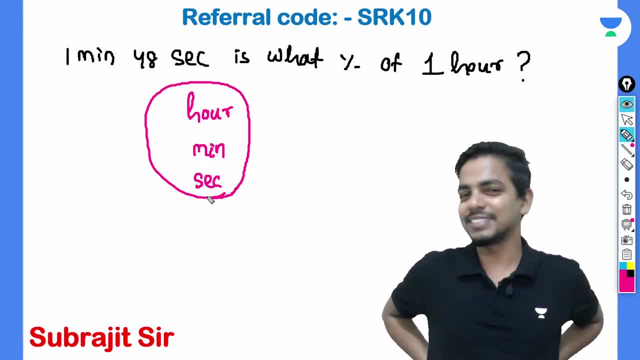 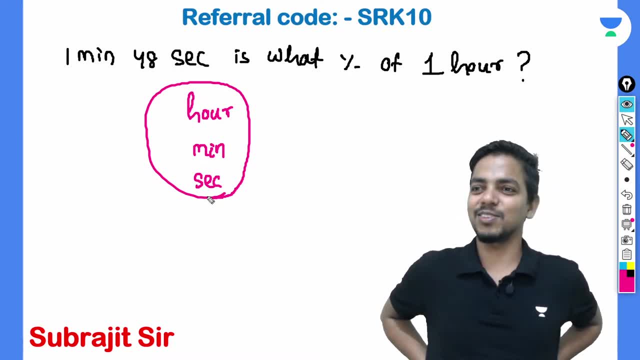 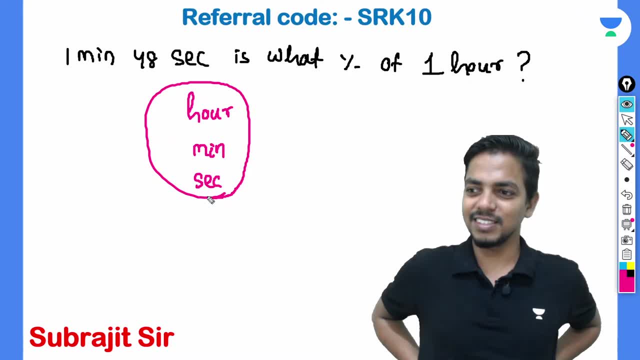 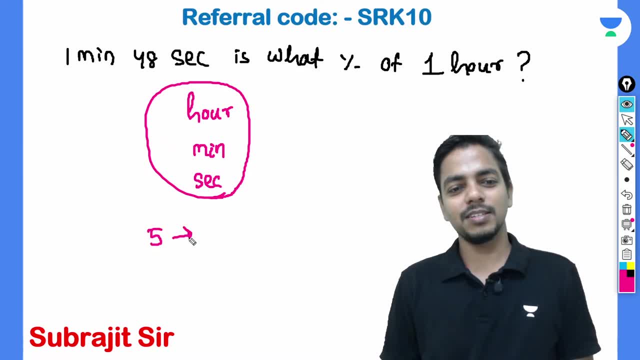 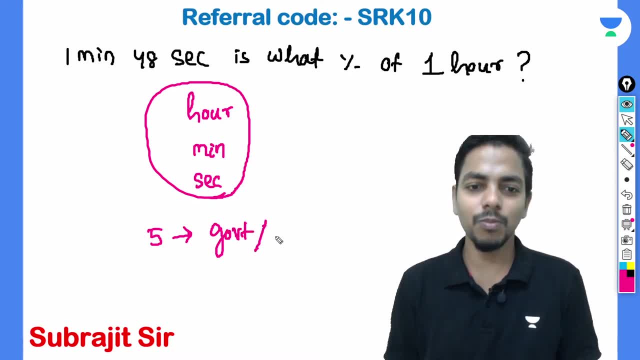 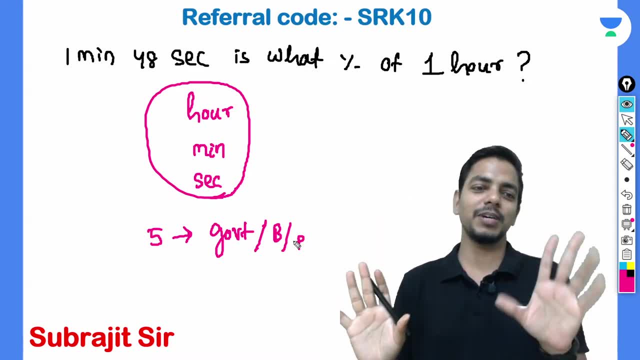 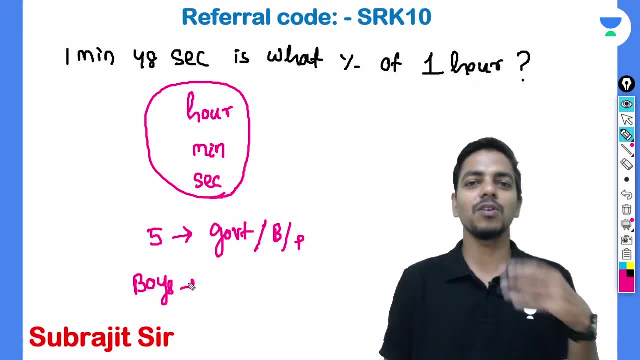 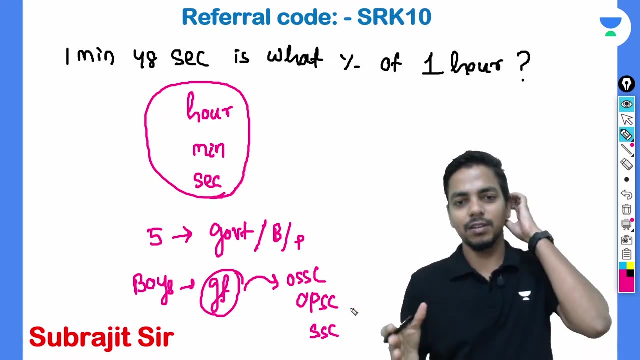 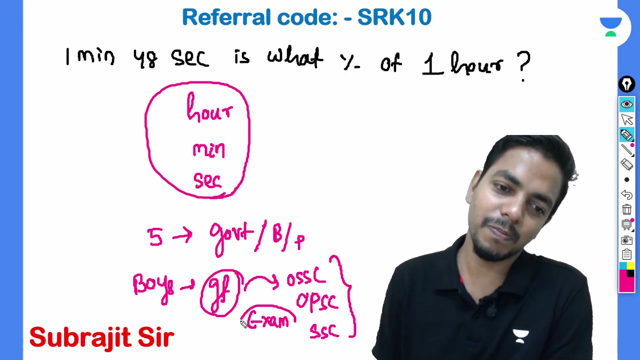 you will be seen in front of the audience. you will be seen in front of the audience If you are going to get your cross or girlfriend or your dream girl- OSSC, OPSC, SSC, Army, Navy, CTS- you will have to prepare for all these exams. crack the exam when you get the government job, then you can marry your father. 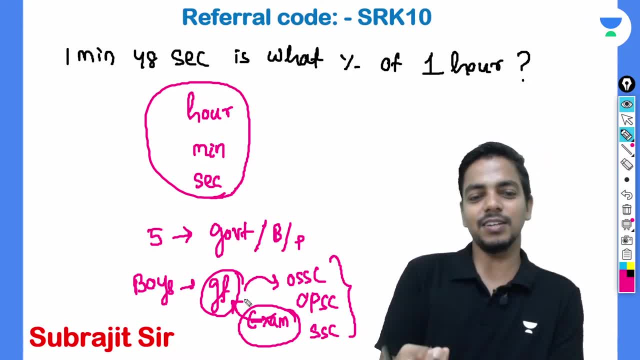 Otherwise, after a few days, the day of marriage will come. someone else will take away your father's gold. your father, your gold will belong to someone else. right? You can say this too: your gold will belong to someone else. then he will say bye-bye, right. 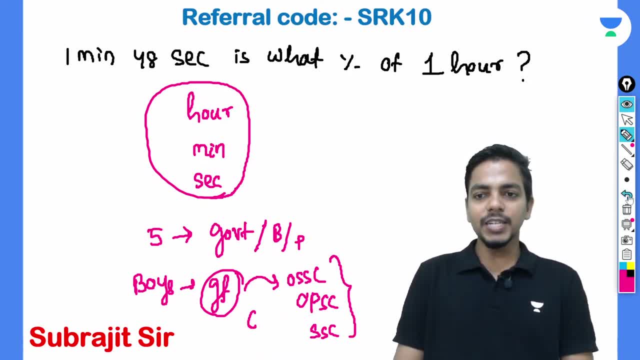 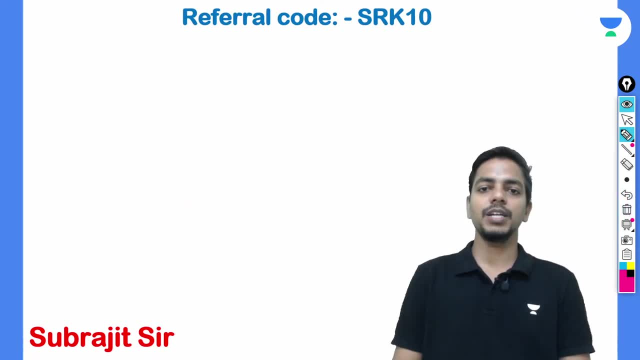 Okay, let's go. 1 minute 48 seconds is 60% of 1 hour. How will you do this? Give the formula X is 50% of Y. I will write the question: 1 minute 48 seconds is 50% of 1 hour. 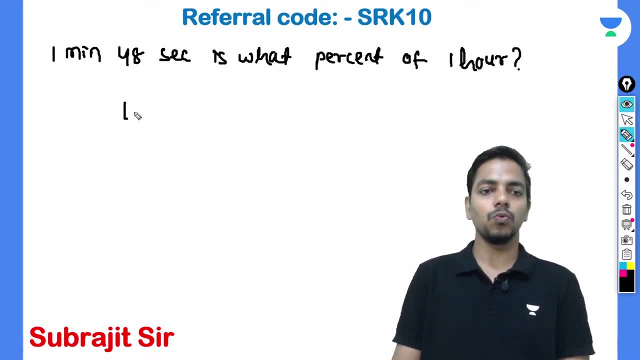 How will you do this? 1 minute 48 seconds divided by 1 hour, 1 hour into 100.. Isn't it? Isn't it? Listen? Oh, the minute is different, the second is different, the hour is also different. 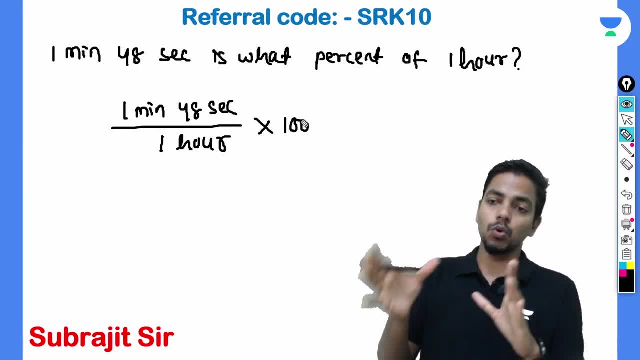 You will convert that All of them are less units. That's why it was said that someone standing down will fall, sometimes 48,. 48 seconds is good. How many seconds do you have in 1 minute? In 30 seconds? 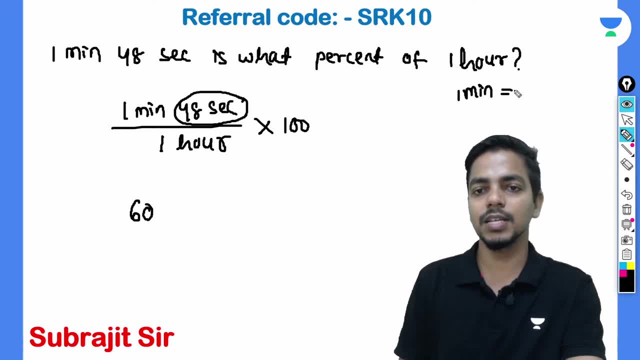 second: like you do one minute, get the second. now set the second. come in, kid. you set your plus or a choice: one hour, get the second of one hour. I'm paper, you go. so this is so. second, set your plus or charity divided by. so this is so in 200 today by the boss. so a art a divided by, so this is so in 200. 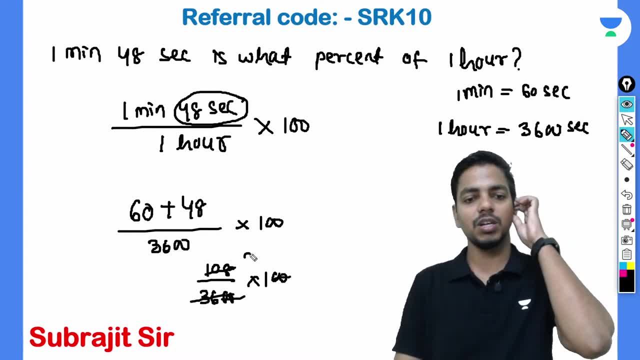 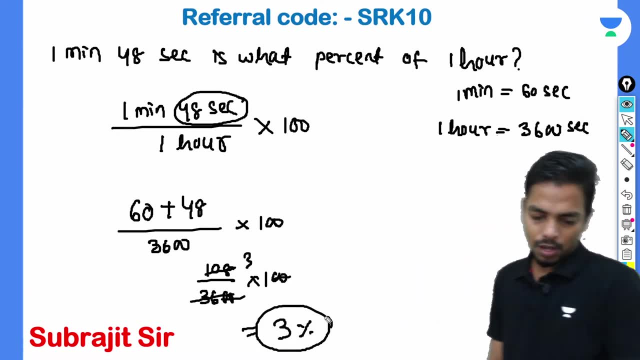 get the cartridge details on the details on the particular. so this is theory negative, so theory. author of art retina. like a thing to know about us. three percent as the other more correct answer: the kingdom that I don't have a child, Bob money. the Kenya got out a lot of a chariot football class man under a link. 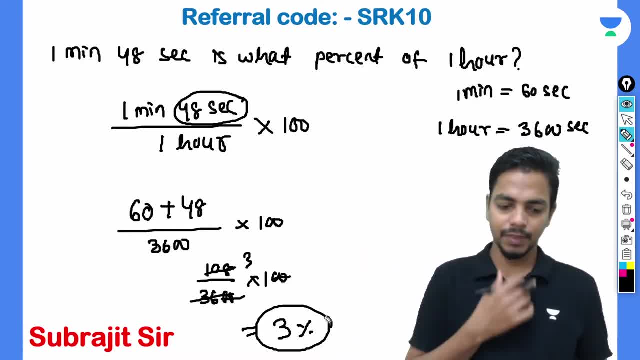 to the million a message for me. give up next questions. could you back tell me you tomorrow, fast part of our percentage of the chapter pastor, part right, certainly one hour. we want to think under a class in a given good, a good, a minute. new cella, cella. 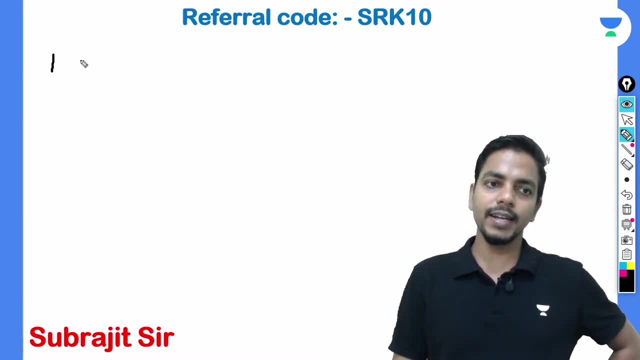 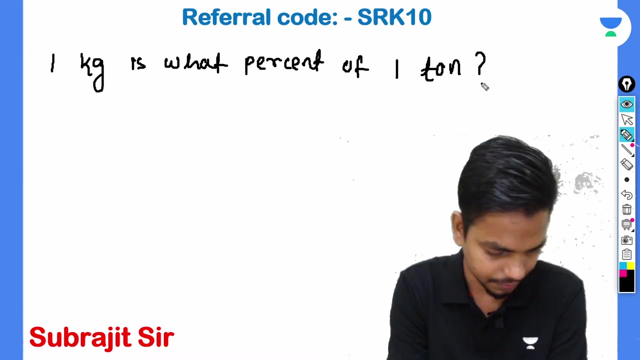 who did it. I'm quick way. he won. k3 is part percent. Oh one, so go number a message for you, sir. please go with them. they are double nice if I have a great calm time to class and I'm going to but continue by one one minute. sorry, one page is part percent of one time that I told the 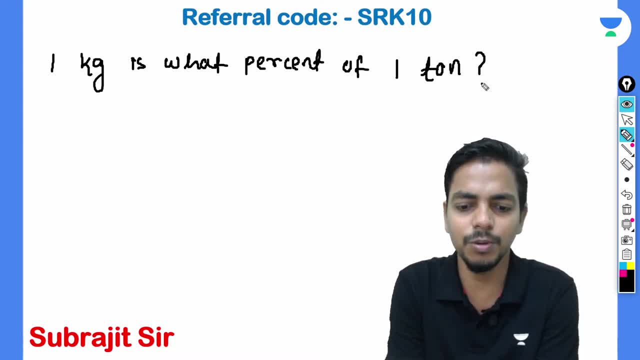 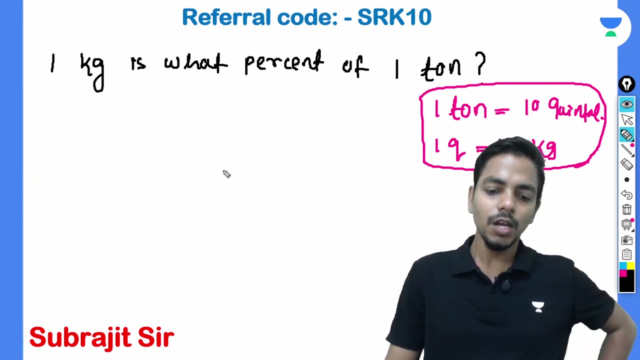 answer. don't tell you can move on. so they've been out. huh, maybe the exam, the war, huh, the side of the kid. they are formula. he won't. 1 ton is equal to 10 quintal and 1 quintal is equal to 100 kg. you can say 1 kg divided. 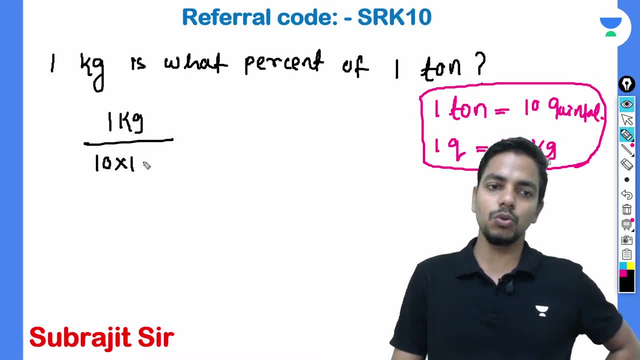 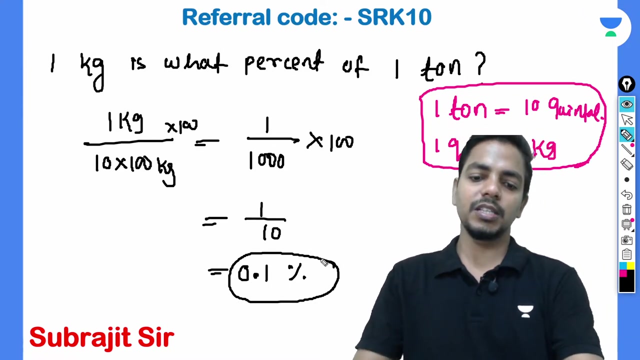 by 1000, which is 1 ton of acid. 10 into 100 kg of acid, which is 1 kg. divided by 1000 into 100, which is 1 upon 10, which is 0.1% percentage. you can see the doubt is there. 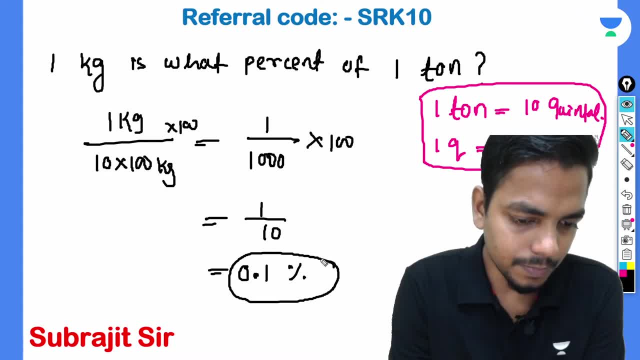 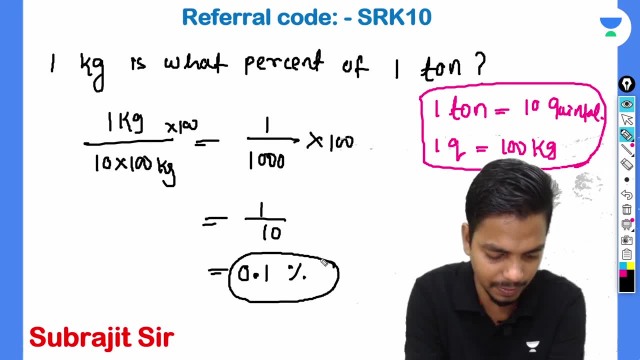 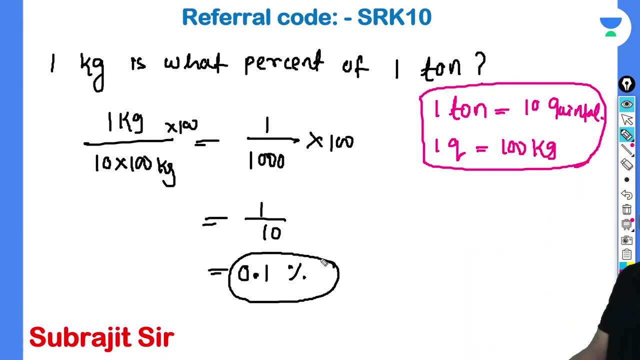 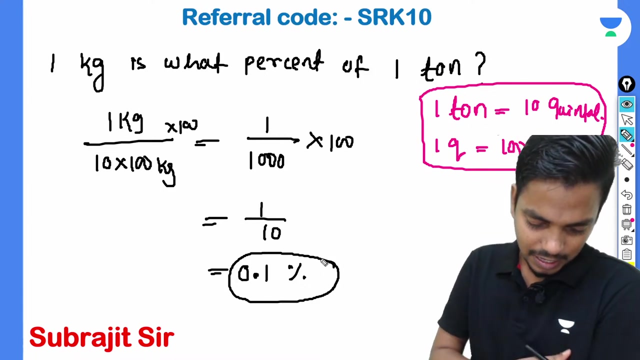 right. My teacher can pay even 100, he has a very good competition. he will take his child or 5 tons and then he will sell them to get at a satisfied price at 2,000.. Didn't they get a lot of 0.7% this year? in this year, for pandemic group, schools are 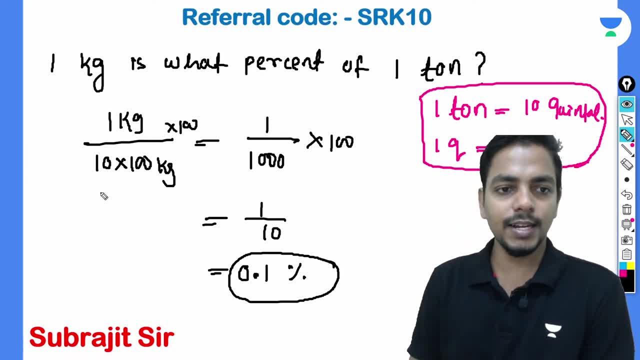 also doing well. M doin a lot of good work. If you had given a formula, you would have been late. This is the problem. If you had given a formula, you would have been late. If you had given 5 times the time, you would have been late. 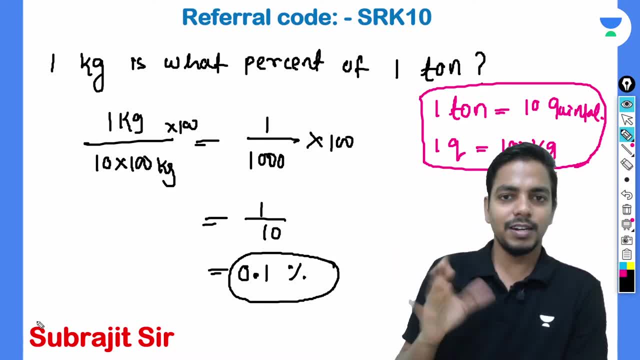 Our class is also here. You have to give the class time. You are late. I gave you a formula: x is 4% of y, x is 4% of y. You can give x upon y into 100.. Same thing. 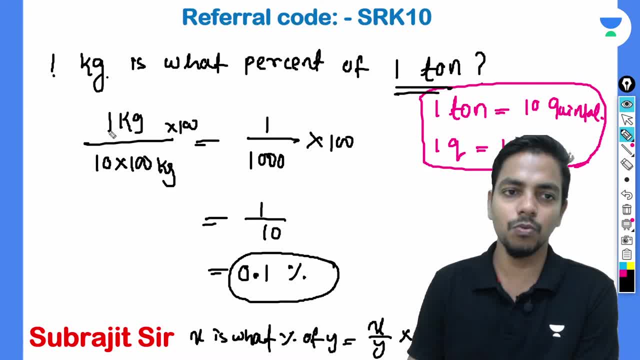 1 kg is 5% of 1 tonne. You can write: 1 kg divided by 1 tonne, The result is 1000 kg. Calculation is 0.1%. Calculation is 0.1%. That was the introduction class. 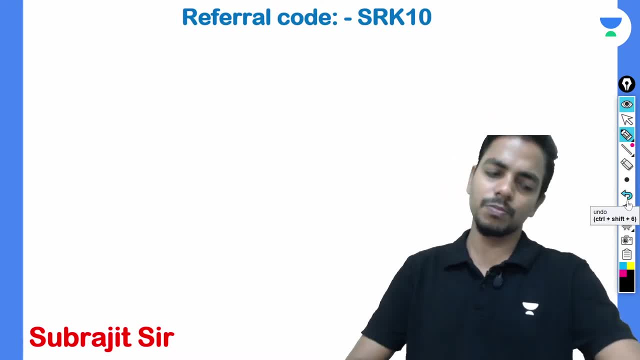 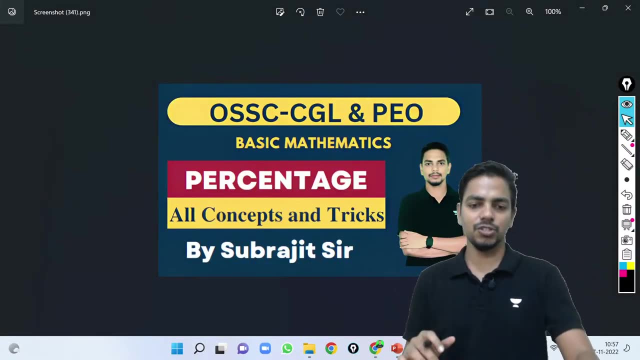 You are still late. You are cat is snowing. I have completed the syllabus. You need time. I just let you know that I am starting a session. I just let you know that I am starting a session And what do you think of the problem? 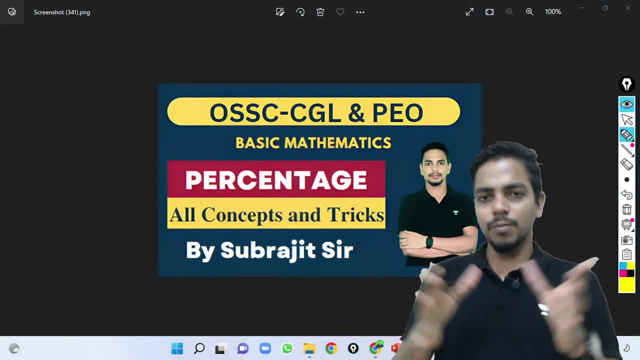 This is actually our online class. As you all know, we have a class on YouTube, So you can see this online class. I can hear you, But I can't hear you either. I don't know if you will get any message or not. 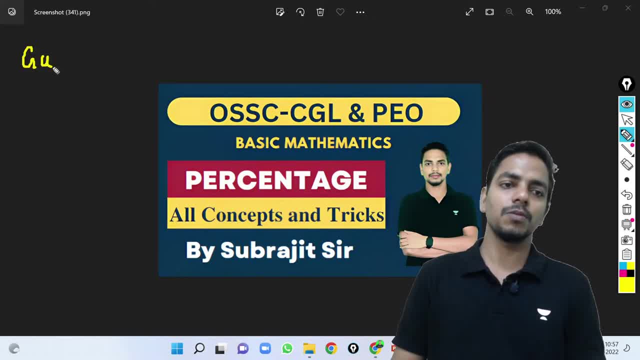 So there is nothing to see. You have to give some guidance. What do you think If you have OSHC, CGL and PEO? give them some guidance. Whatever they tell you, you will read it. Which material will you read? 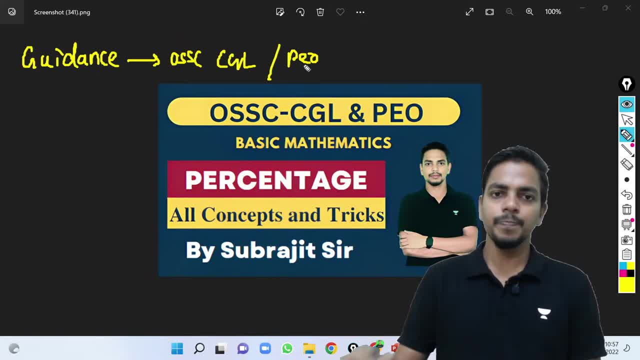 Which selection will you have? You will know this information. This will be every Sunday And we will do this directly. We will help everyone, Whether it is on Zoom or Google Meet. We will do this. Everyone can join this. You can pay here. 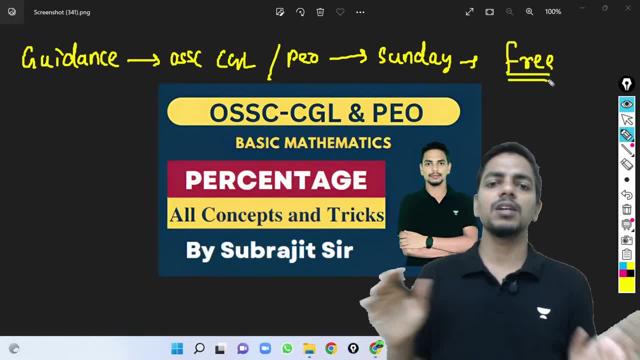 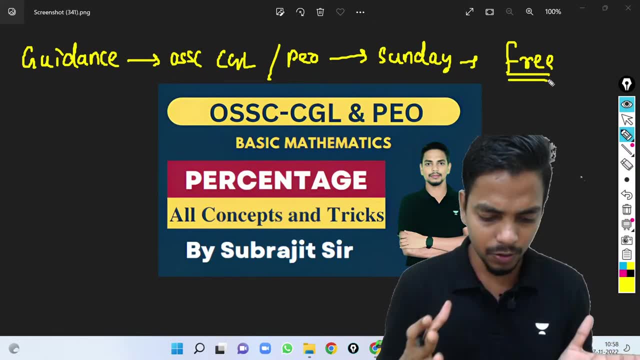 You don't have to pay anything, Totally free. If you have any financial problem, Or if you have any financial problem, Or if you have any money problem, You can't get any subscription. You will be happy to know this. You will get guidance for free. 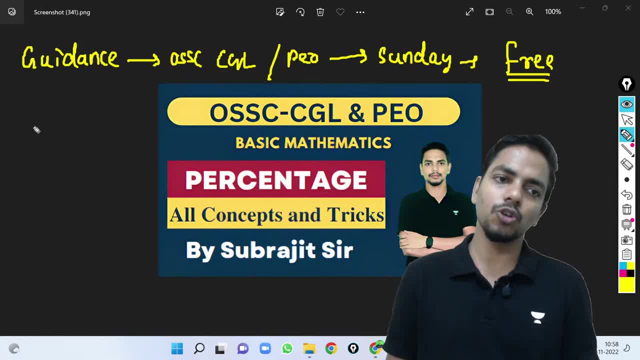 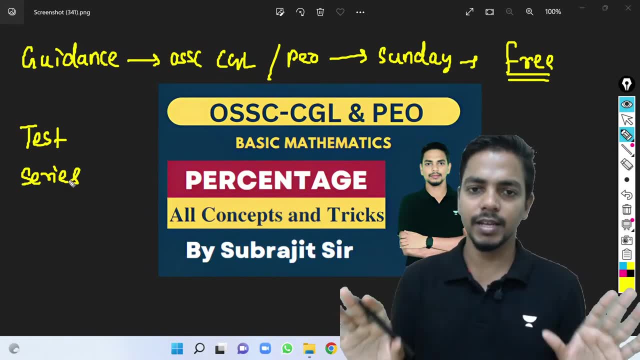 Even then, next week We will do a test series. for all the weeks Your test series will be free, No payment. How can you do this? You have to search it and send a message. The date will be free As long as there is call. 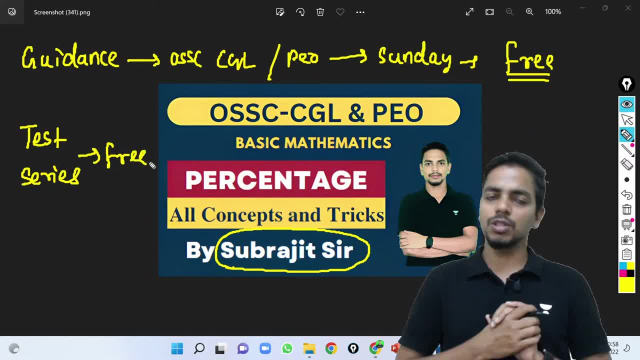 It will be free. If you have any doubt, There is a call, There is no need to message. I will reach you with this. You will give the free. You will meet on Google or Zoom And I will provide it to you. 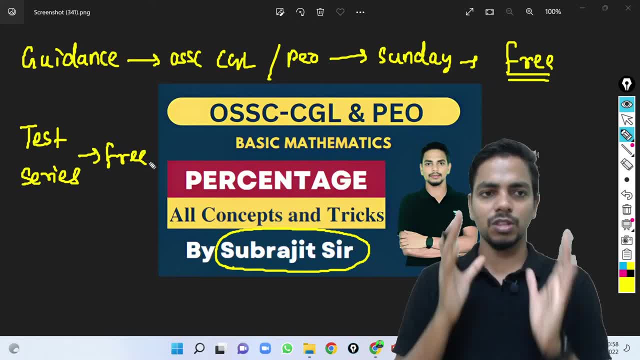 I will hear from you. I will provide guidance. It is totally free. I will be in the test. Only Bhubaneswar Pillai. I am getting such guidance. You can get the same. I am getting the same. Are you getting the same? 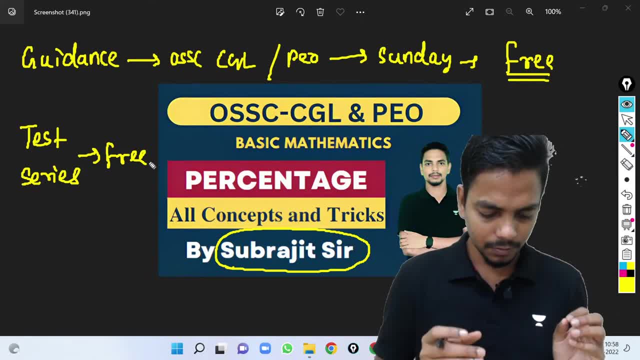 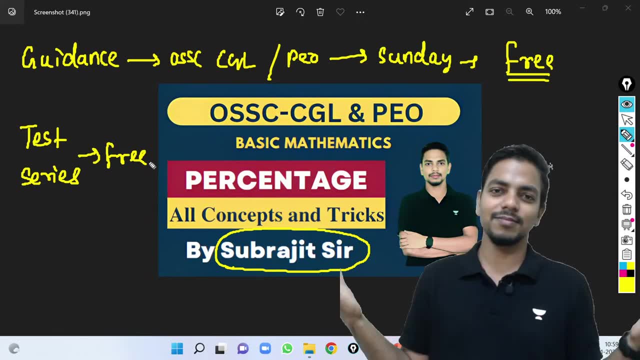 Today. It is expired. I am getting it, You can get it, We have, We have. We have all the time, We have all the time. Don't worry, I am a big fan of Sambalpur Pillai Sambalpur Ballet Show. wherever you are, you will be free. you will be able to do a lot of work. 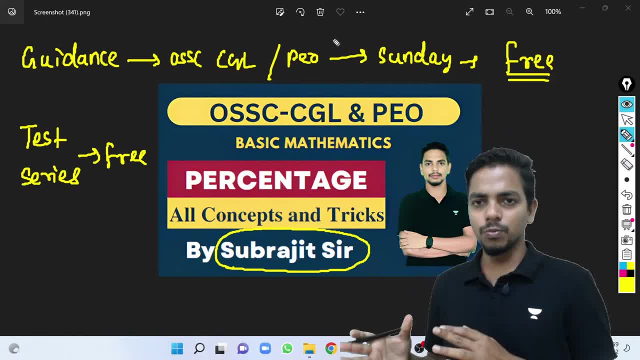 Join us on Sunday on Google Meet or Zoom. you will be totally free. there is no payment. you will be totally free, even if you get the same. you will be able to message Subrajit Sir. otherwise you will be able to get whatever you search.